What do you make of this? Five, six, re re. What do you think comes next? I'm gonna go seven, Seven, No, actually it's another three. Now you have a guess what's coming next? Three, Good, yes, As a matter of fact, it continues to be three, three, three. And you wonder? this is 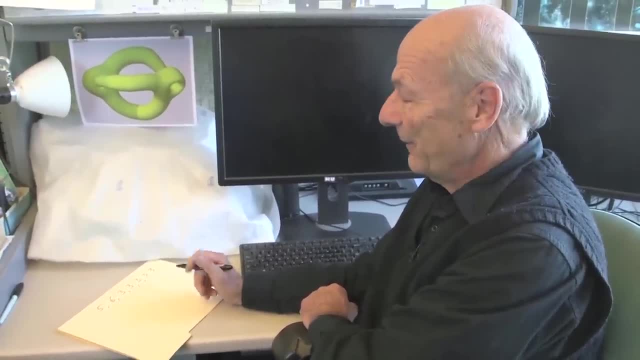 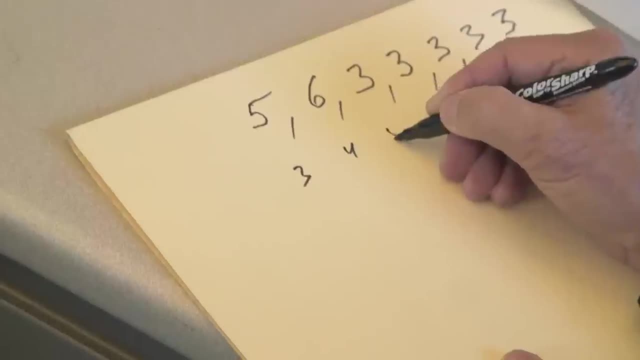 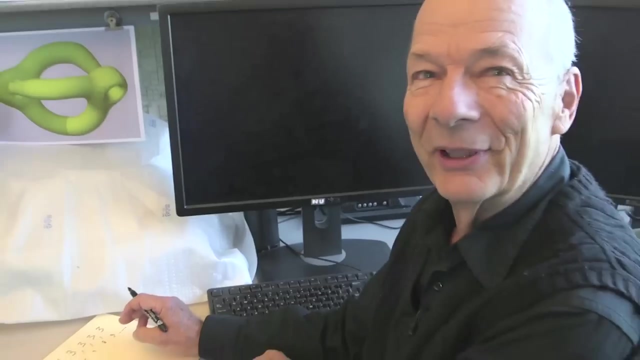 really a strange sequence. you know What are we going to do with this? Well, this is the number of regular polytopes that exist in three, four, five, six, seven, eight, nine and all higher dimensions. And that's what we're going to talk about today: Regular polytopes and then dimensions. A polytope- 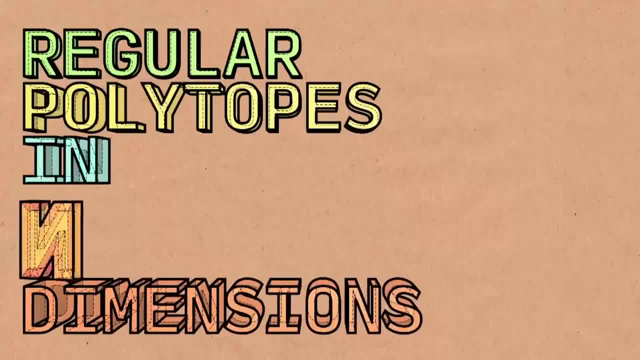 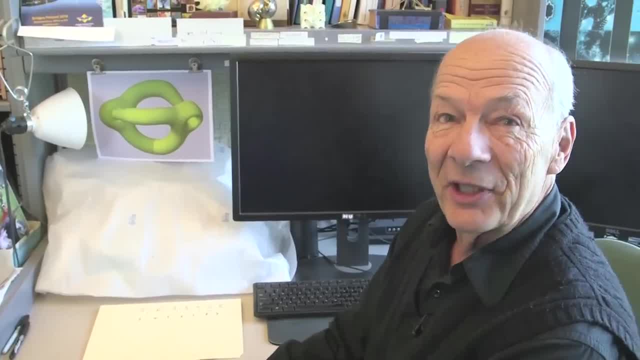 is just a more general term that generalizes from two-dimensional polygons, three-dimensional polyhedra and everything higher we call a regular polytope. That sounds a little scary, so let's start with something much simpler: the platonic solid. So here is a tetrahedron. That's the first. 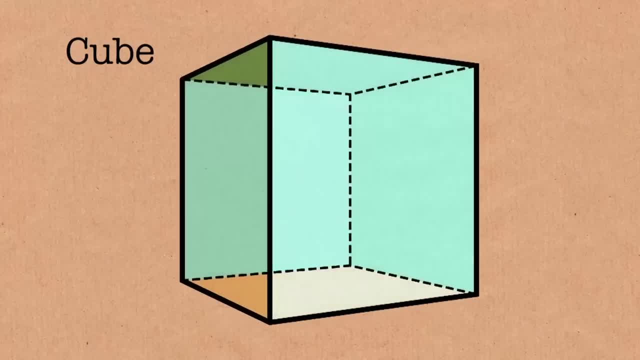 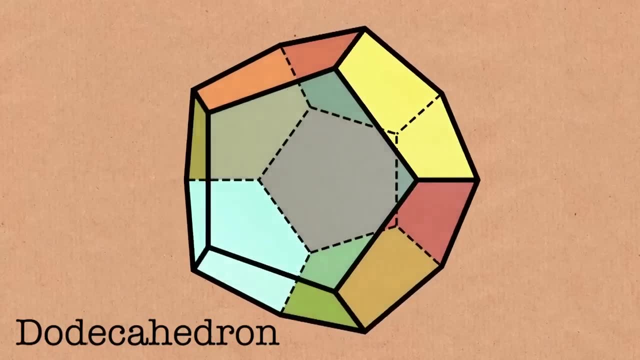 platonic, solid. Next, we have a simple cube, Third one octahedron, made from eight equilateral triangles. Number four, twelve faces the dodecahedron. This one has 12 pentagons And finally, a real jewel. 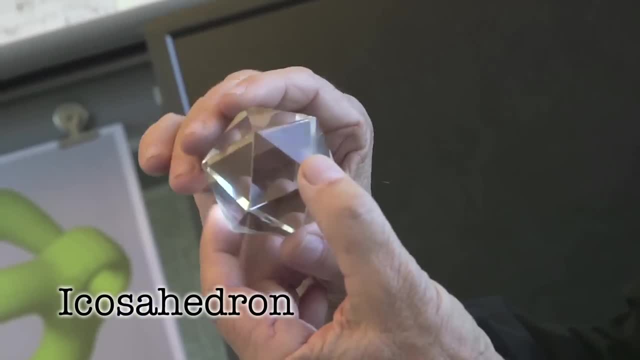 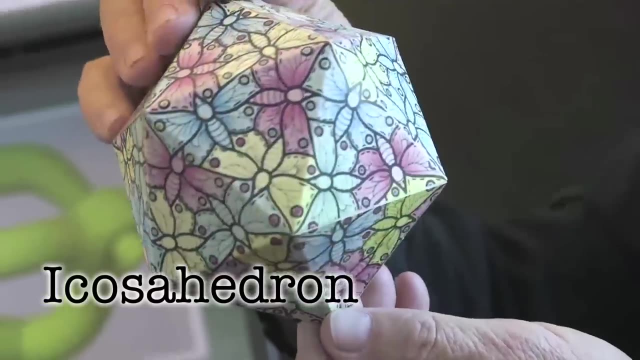 the icizahedron made out of 20 equilateral triangles And this is probably a Swiss crystal. And here is another view of an icizahedron. This is a pattern by MC Escher. Could you show to a non-mathematician in an intuitive way why? 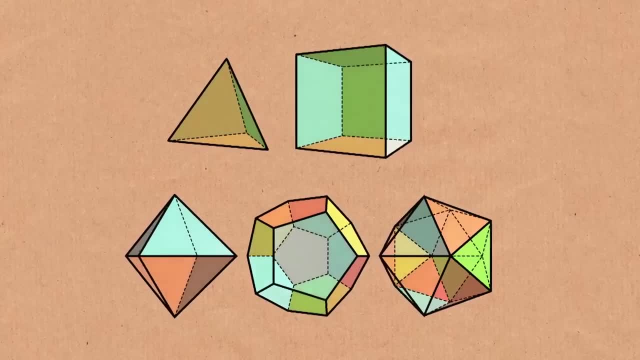 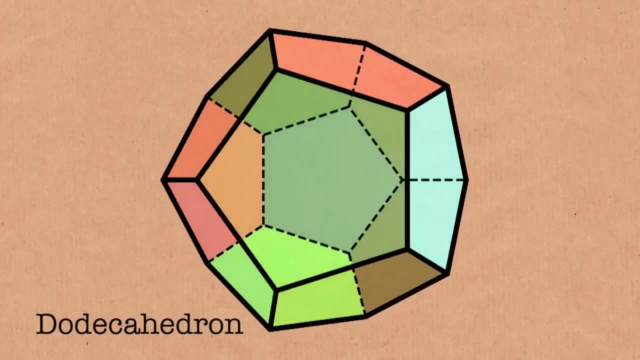 there are exactly five platonic solids, not more and not less. Well, one way to do it is to look at the surface of these objects. So this dodecahedron, for instance, is made out of regular pentagons. 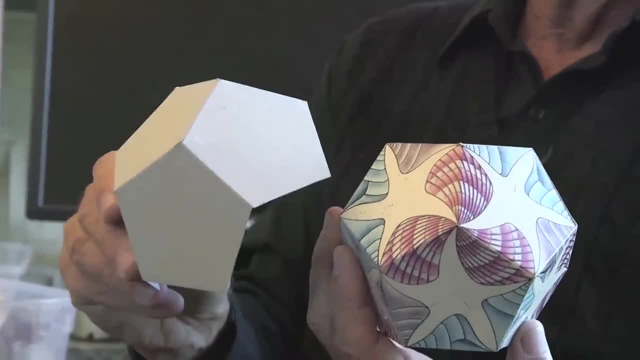 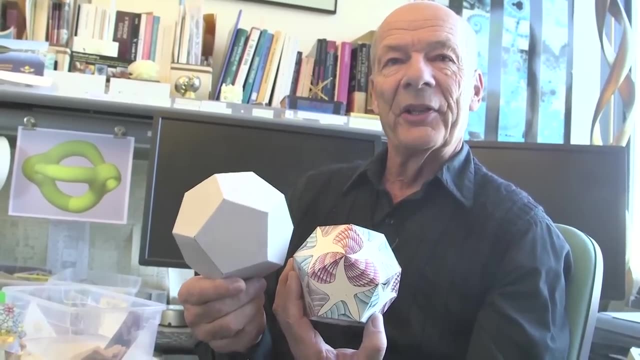 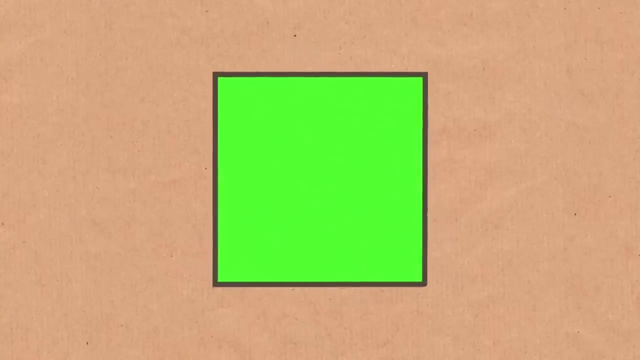 And so all of these platonic solids are made out of regular polygons. So probably we should step down a dimension and look at what regular polygons are possible. Simplest one, this would be a regular equilateral triangle. Then we can do a square, Then we can do a pentagon. 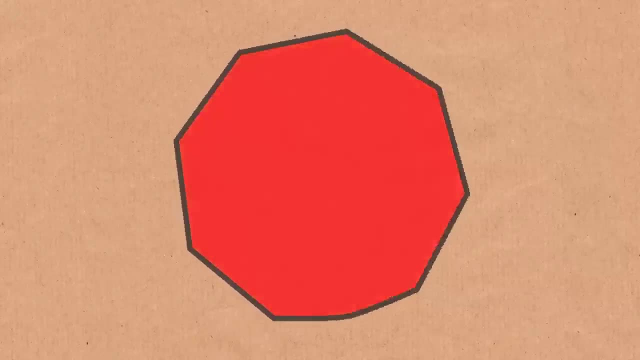 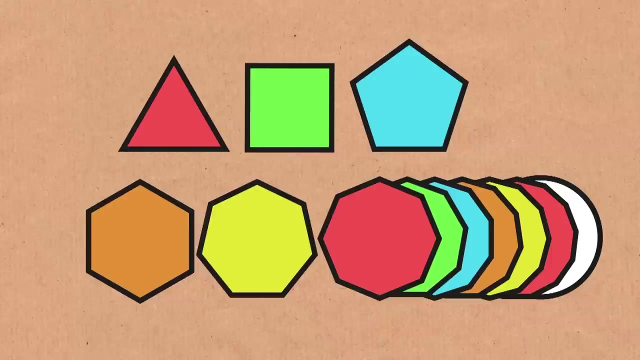 Then we can do a hexagon and so on, And if you go all the way to infinity we end up with something that looks like a circle. So there are infinitely many of these regular polygons in two dimensions. So really the sequence up here it has another character before the five, if you go to two. 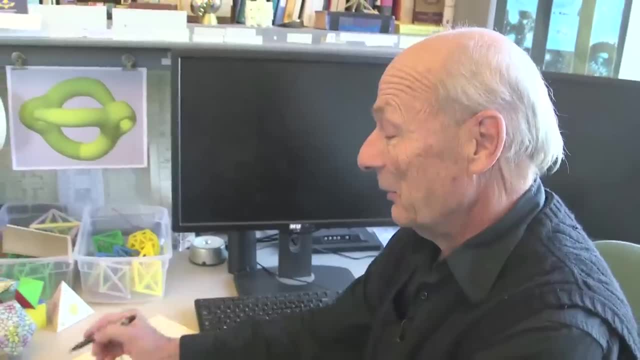 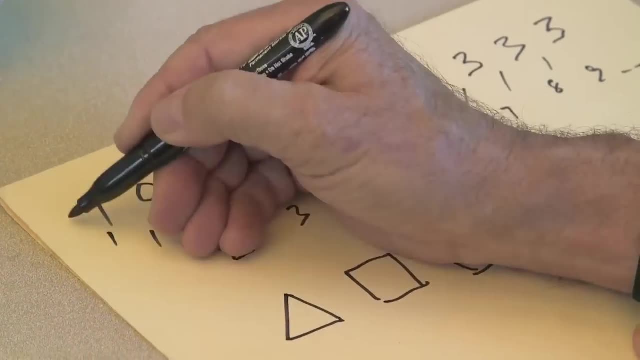 dimensions, And what's that? It's not an eight, it's infinity. And if you really want to go to the extreme, what about one dimension? It's just a line segment, nothing else. What about zero dimension? Well, it's just a point. 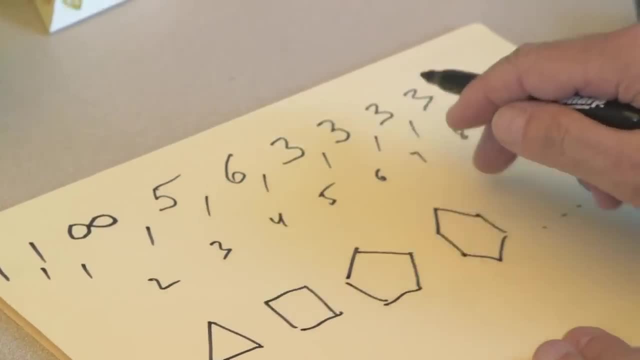 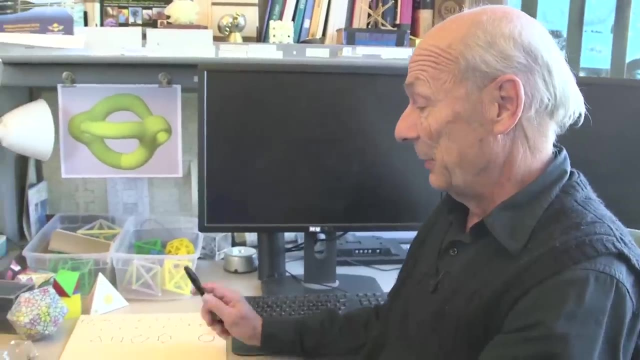 nothing else, But now one one, infinity five, six, three, three, three, three, three, three. That's a really weird sequence, you know, And I guess I would really confuse people. Okay, all the platonic solids. 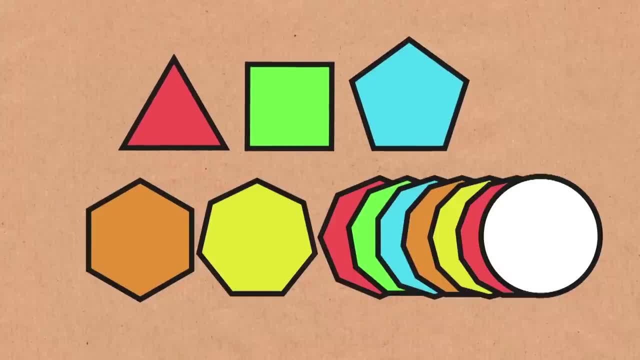 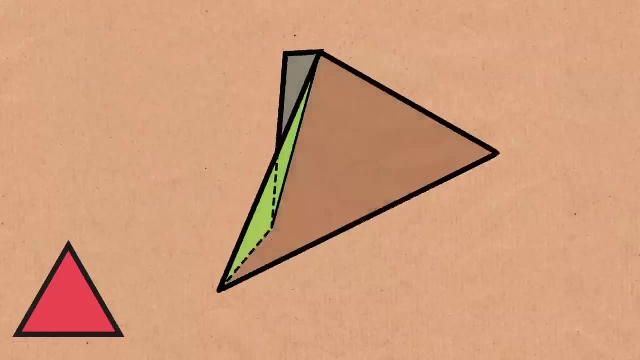 are made from one of these regular polygons. And so how many different ways can we use these regular polygons to make one of these solids? Start with the equilateral triangle and ask: how can we make it out of that one? Well, we need a minimum of three of those to be put around the corner in. 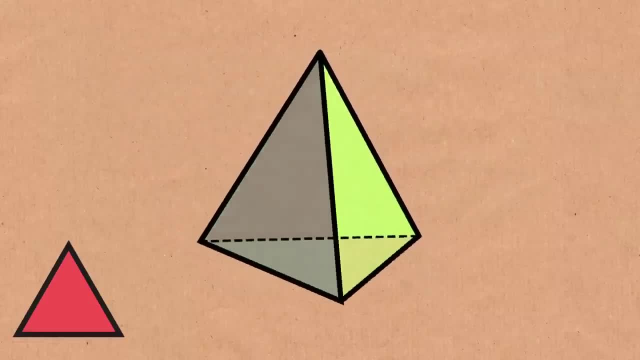 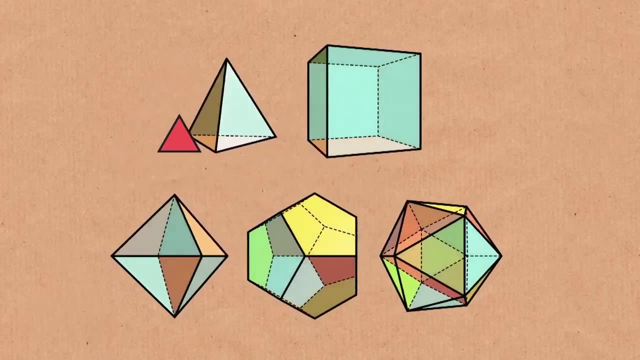 order to make a valid corner in three dimensions. And if we put three of these triangles around a shared vertex, then the bottom is also an equilateral triangle. That would give us a tetrahedron. Okay, so next we can try to put four equilateral triangles around the shared 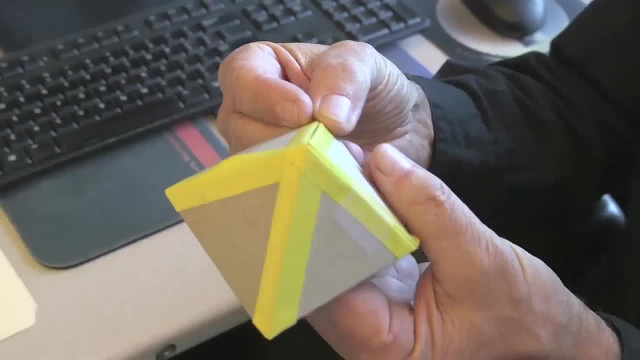 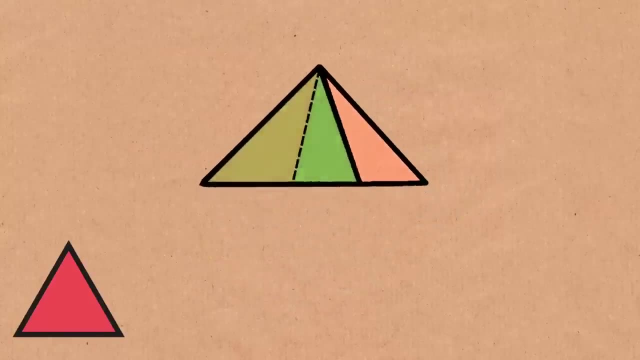 vertex And we can bring them together and make a four-sided pyramid. And remember, to make it regular, all of the dihedral angles here have to be exactly the same. So that means that the bottom now is a point and the bottom is an equilateral triangle And that means that the bottom now is a. 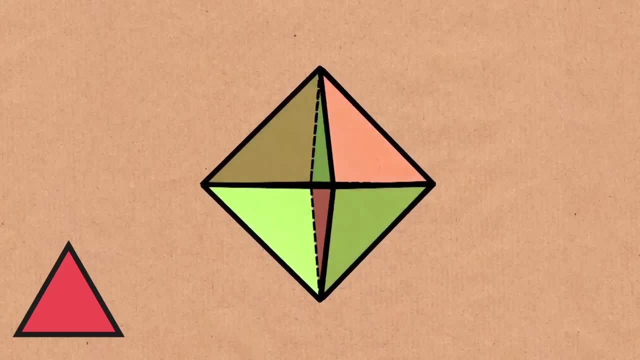 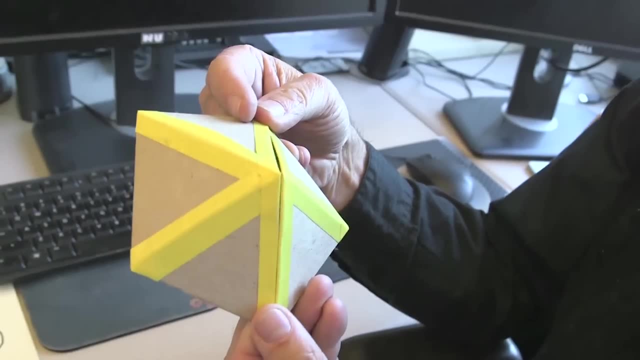 perfect square. We can take this square pyramid and match it with an identical square pyramid, So that makes the second platonic solid, the octahedron. Now we can try to take five of those and put them around a vertex And this makes this five-sided pyramid. So it's completely symmetrical. 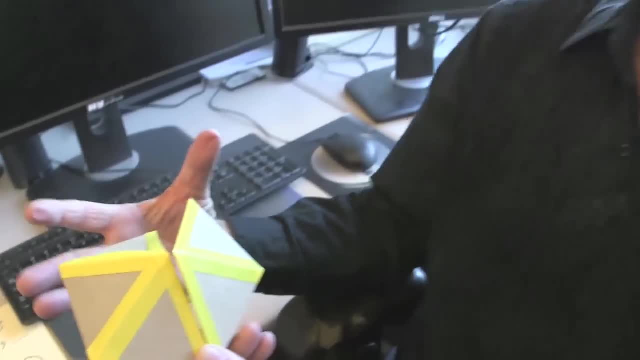 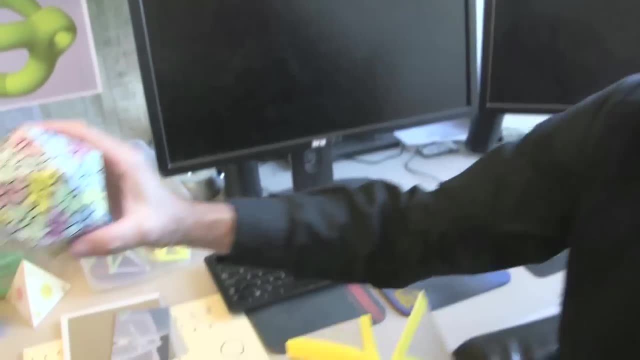 If we continue forming these kind of corners and try to sort of wrap it around, will this actually get the closed surface? Will this actually end up in something useful? Well, we know we have this icosahedron. okay, But if you have to, 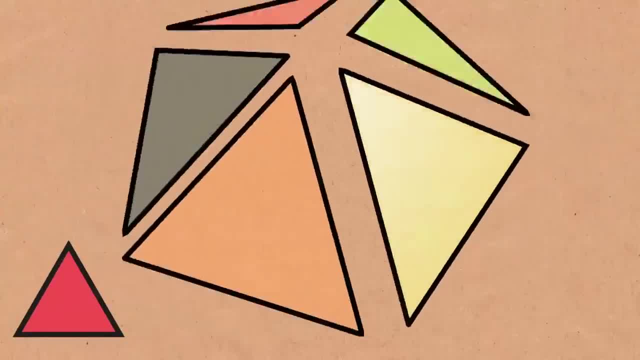 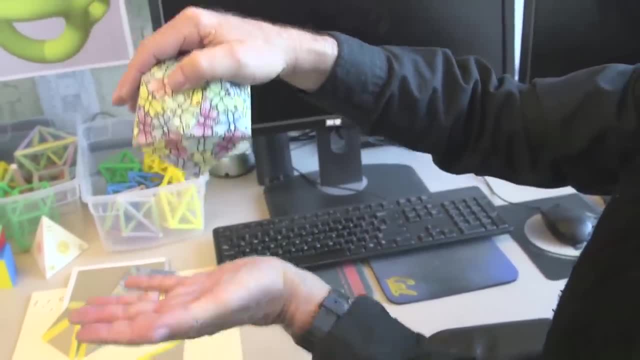 really figure out whether it works. it takes a little thinking. You can see on top, here we have this five-sided pyramid. We can take one of these five-sided pyramids. We cannot put this one just up on a mirror. We can take another one, but the two have to be rotated against one another. 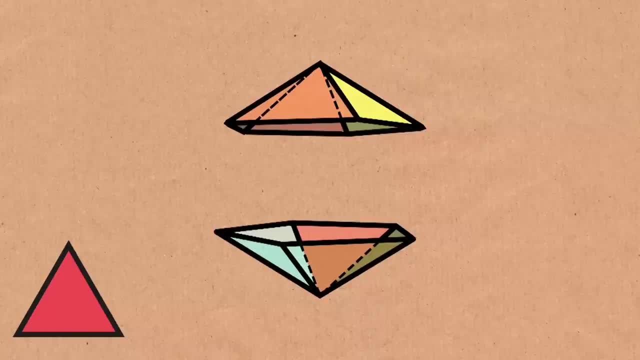 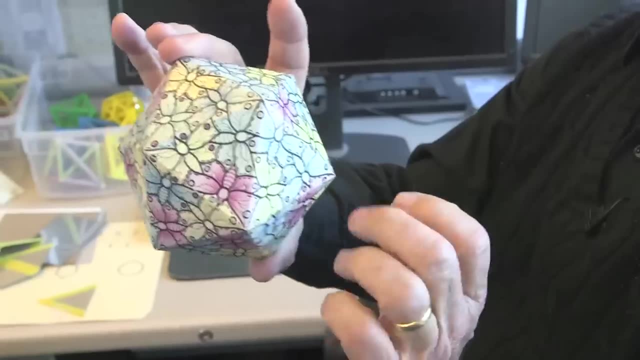 by 36 degrees And if we do that, then in between you can see there's a triangle strip with triangles going up down, up down, up down, essentially forming a five-sided antiprism adding ten more triangles, And it's kind of beautiful that indeed this surface does close and 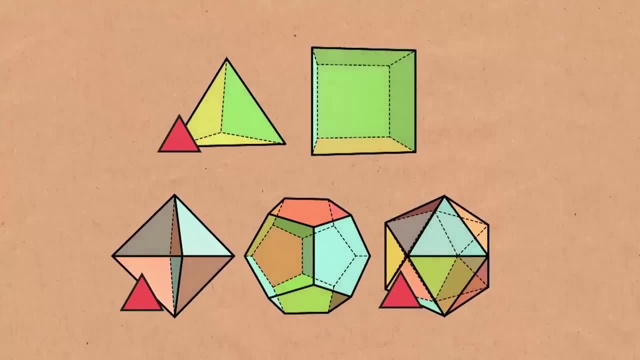 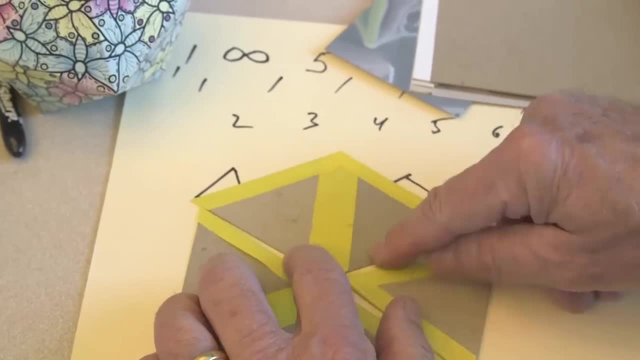 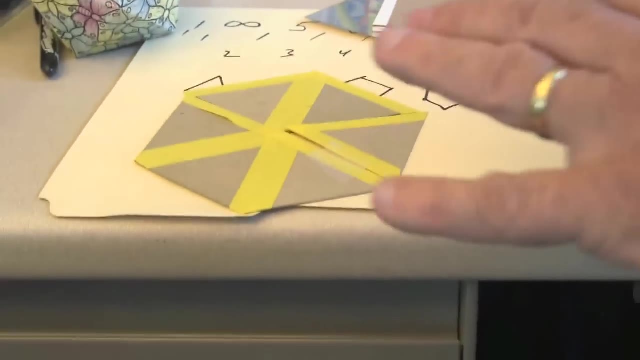 result in number three: platonic, solid. And what about six triangles? Oh, good question, Glad you asked that. So let's try to take six triangles and put them together And we get a wonderful, nice hexagon here. So unfortunately it's totally flat And so this doesn't really curve and it. 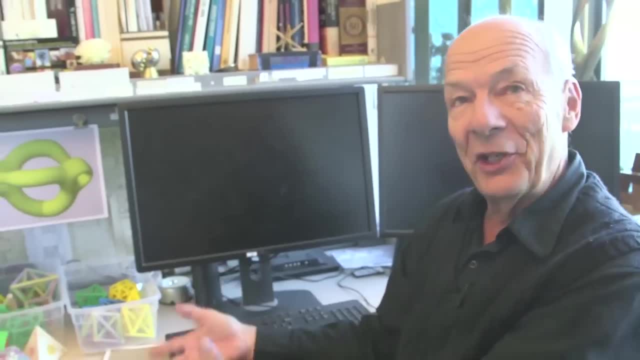 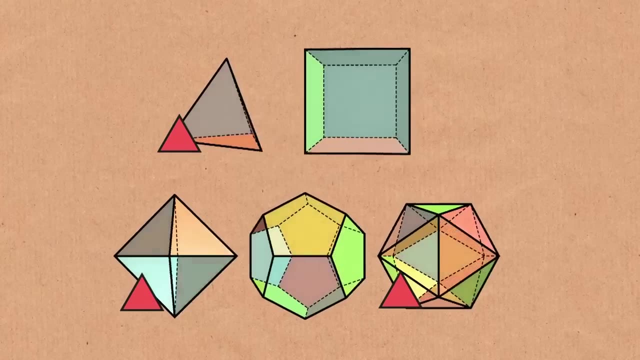 doesn't help you to make some kind of closed object. You can make a kitchen floor with that one. Now, if we go to seven triangles, they don't even fit into the plane. It's kind of get the warped chip and that is no good. So we're done with triangles. So now, 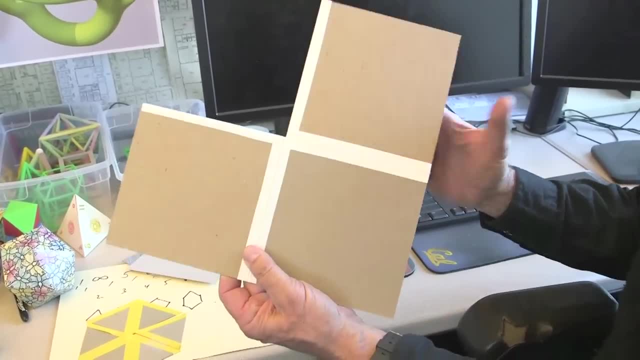 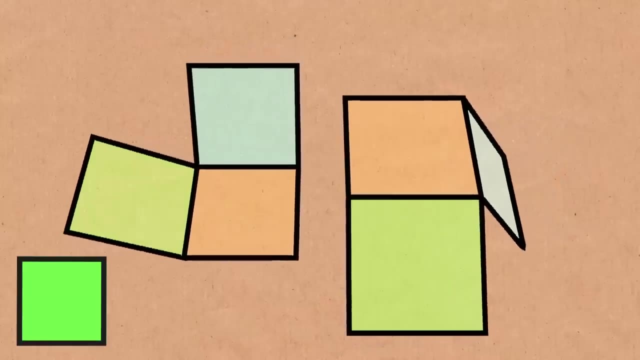 we have to go to squares, Fold them up. So basically three squares around the shared vertex leaves of an opening of 90 degrees And we forcefully try to close this opening And now we have a valid 3D corner. If you take a contraption like that and match it on the 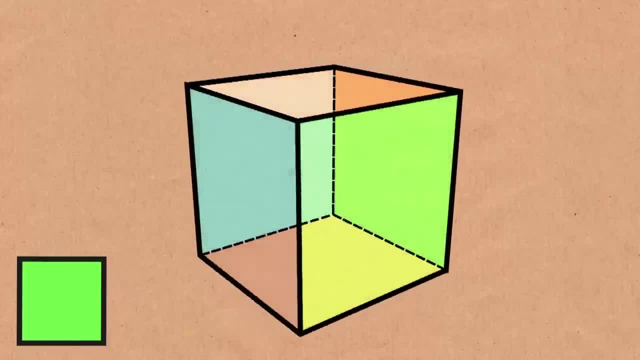 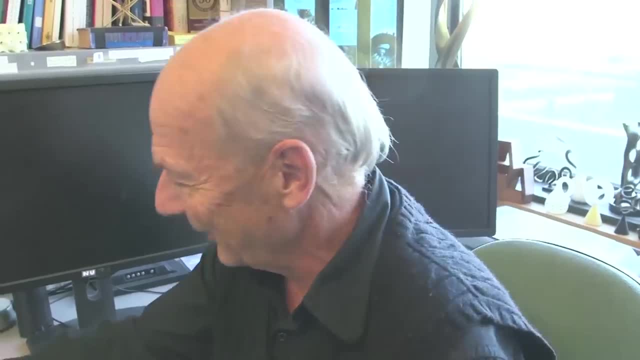 backside with exactly the same contraption. then you get a cube made out of six squares, And I know what you're going to ask next: What about four squares? Well, glad you asked Same problem, Same problem here. So we can put four squares together. 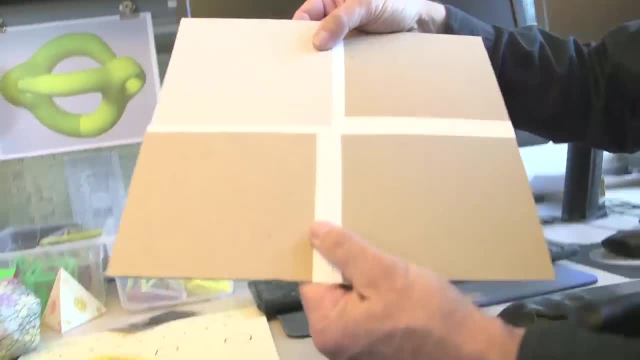 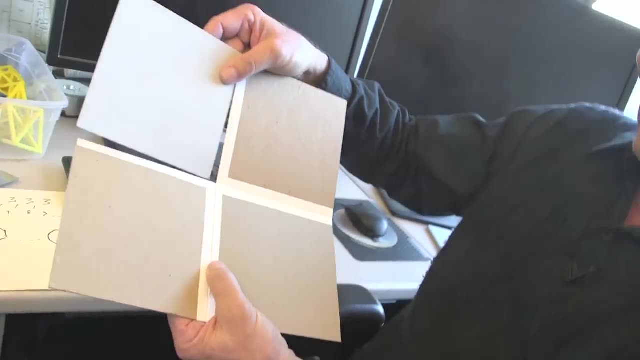 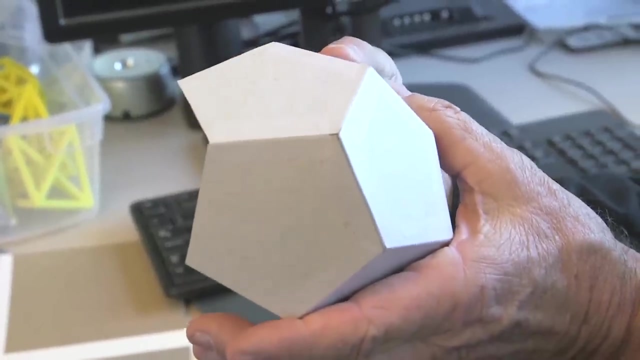 and they make either a complete flat, or if you were to somehow bend it in weird ways, then not all the dihedral angles, at all the edges would be the same, and so it not would be a regular corner that's any useful. So we're done with squares. We can put three pentagons together and 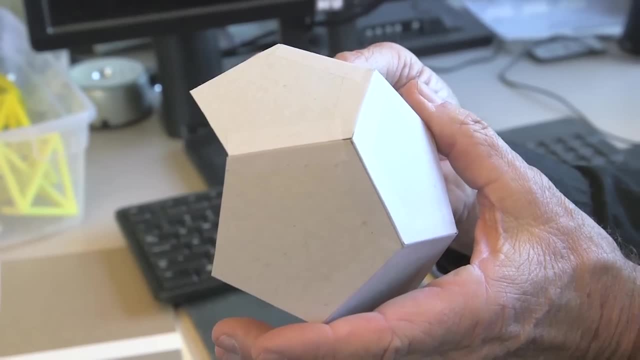 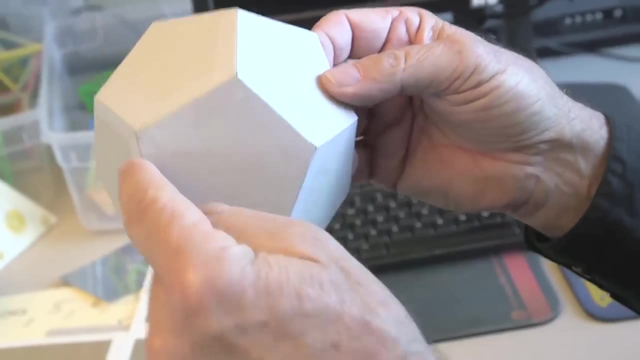 form a nice 3D corner. And again the question arises: does that really close? if you continue the process- And the easiest way to see it is to take one pentagon and put five pentagons around it, completing five of these corners, And then you have a square, And then you have a square. 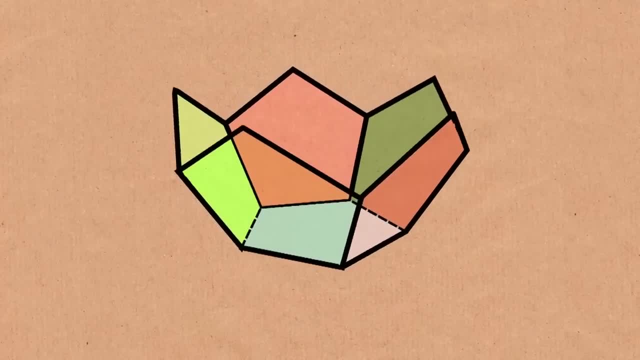 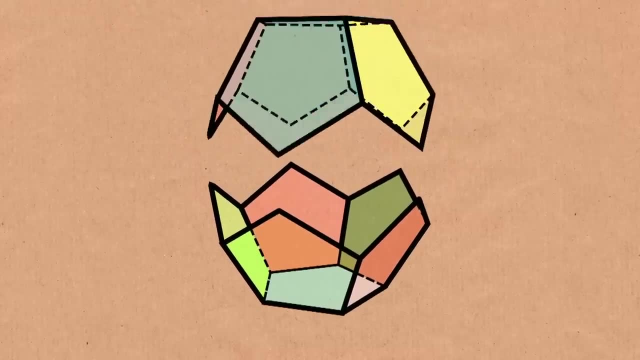 And this makes this nice kind of salad bowl. And now if we put another salad bowl like that on top of it, again rotate by 36 degrees so it fits nicely together, then indeed we can convince ourselves very quickly that that leads to yet another regular platonic, solid Trying to put 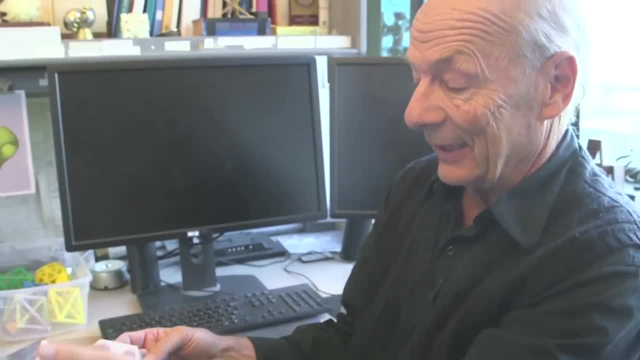 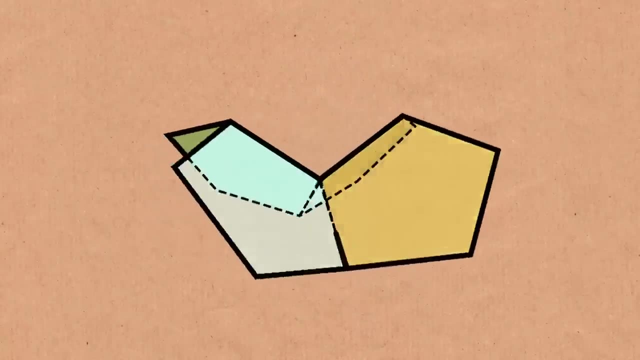 four of these pentagons around the corner exceeds a total of 360 degrees. so you already get something that's warped like a potato chip and it's no good. We're done with pentagons, Hexagons, Hexagons. You know what happens with three hexagons, of course. 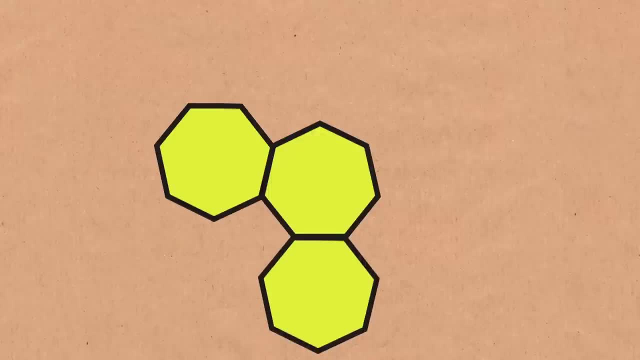 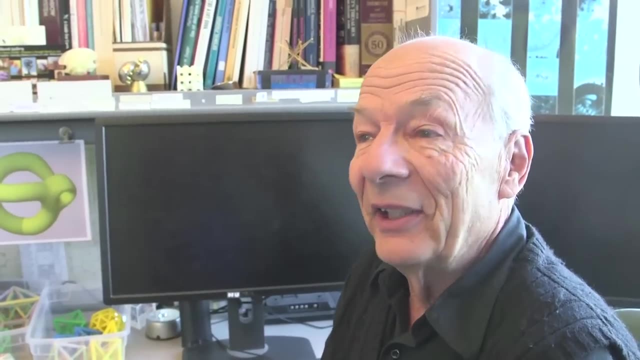 It's a very flat tiling. That's no good. What about heptagons? Well, they don't even really fit into a plane. That's too much. So from there on up, we're sort of done. Nothing new can happen. And now you know exactly why there are five platonic solids. 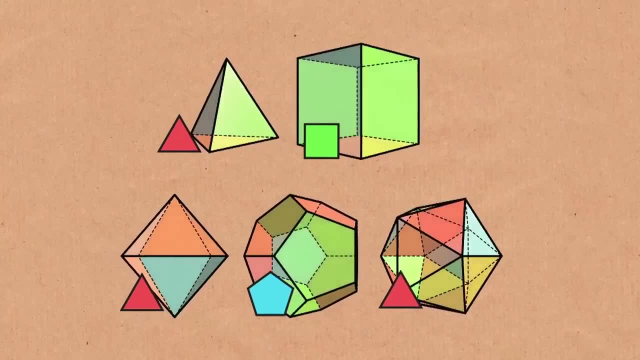 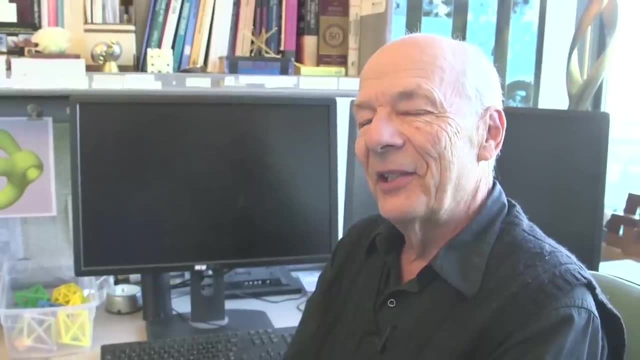 and exactly five platonic solids. Professor, is a sphere a platonic solid? No, it isn't, Because even if you think about a very fine tessellation, you could not find a tessellation on a sphere where all the faces would be exactly the same. 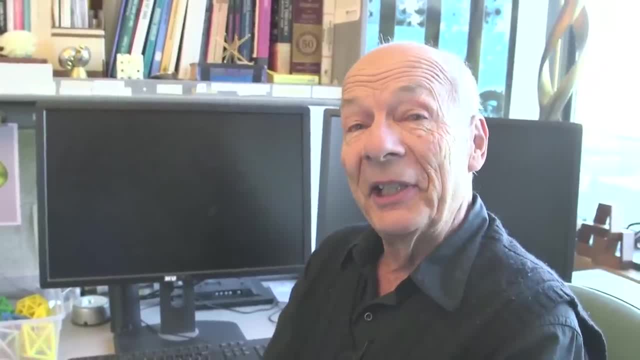 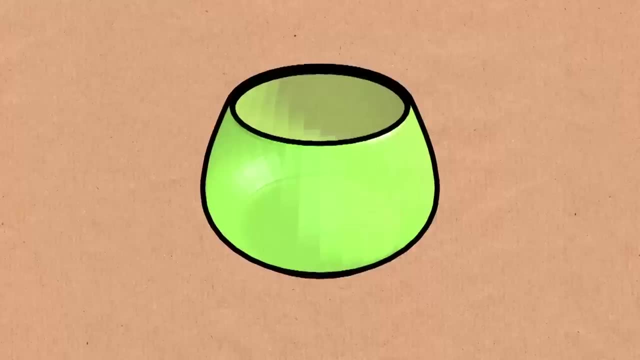 and all the edges are all the same and all the vertices are the same. So we're basically done with three dimensions, And so I must admit that for many of us there's indeed a sixth platonic solid, And it is the Utah teapot For the people in the computer graphics community. 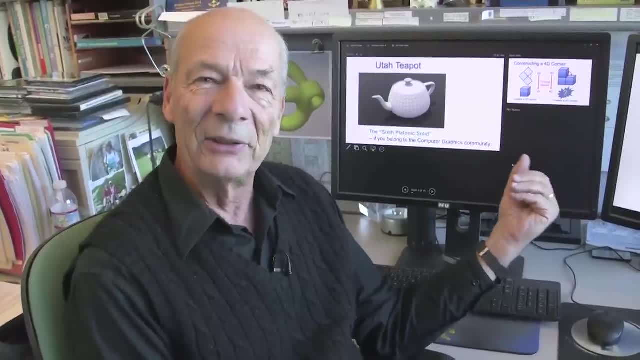 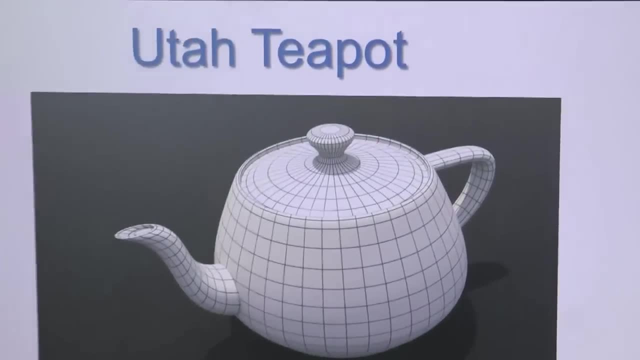 this is such a famous object which has been used again and again to test out rendering software and solid modeling software, And it just shows up in just about every SIGGRAPH paper in some form or another, So we like to think of it as the sixth platonic solid. 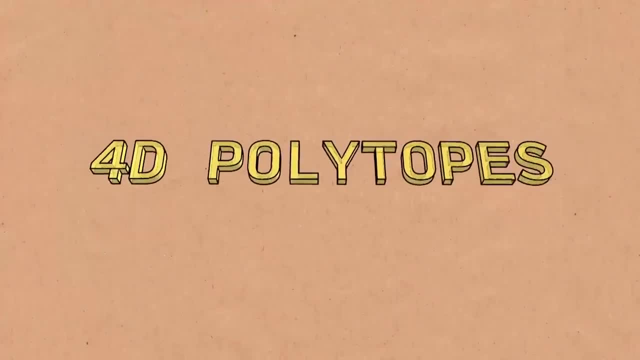 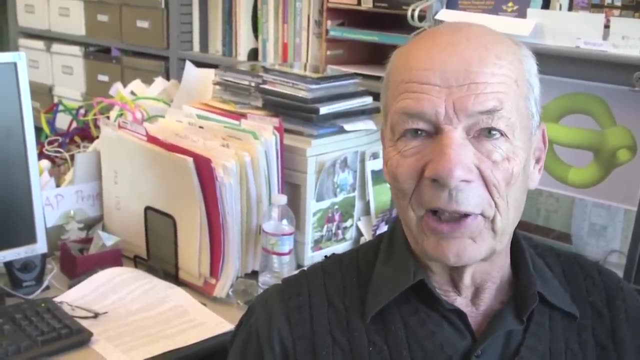 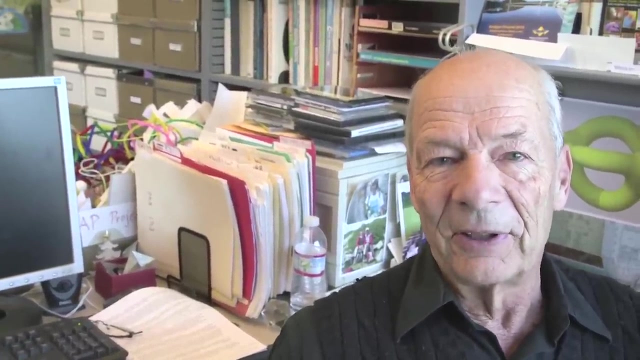 Now these regular polytopes are made out of regular polytopes one dimension lower. In the same way that we made platonic solids out of 2D regular polygons, we can now try to make four-dimensional regular polytopes out of three-dimensional platonic solids. 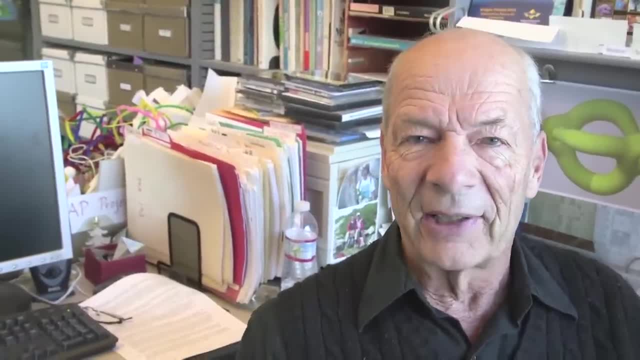 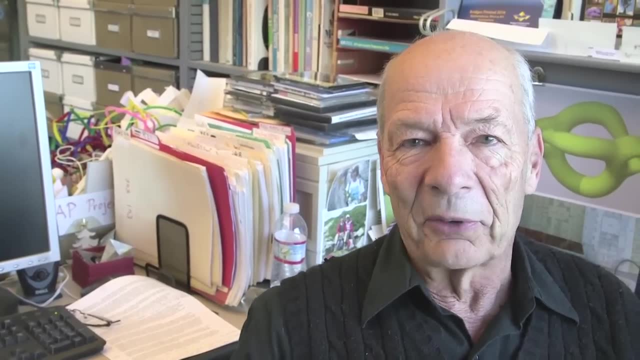 Each one of these four-dimensional regular polytopes is of an object that has as a surface a thick crust of three-dimensional platonic solids. And just like we made a cube out of squares, we're now trying to make a hypercube out of cubes in its surface. 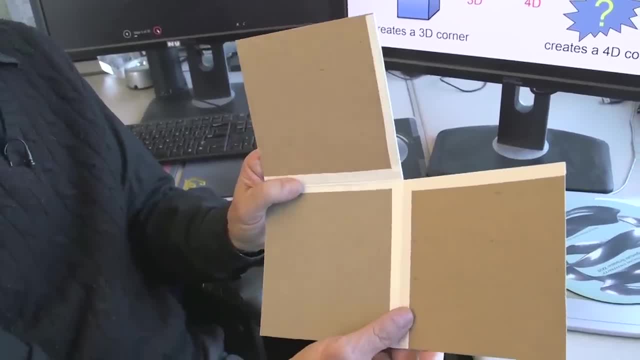 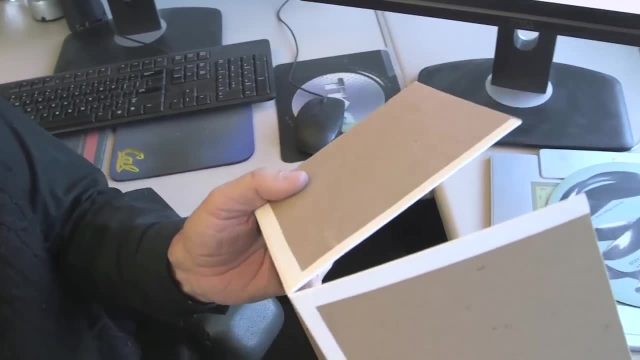 We used to take three squares and then forcefully try to close this gap of 90 degrees, And by closing it we force this corner to pop out of two-dimension, become a three-dimensional, valid polyhedral corner, And that's the corner of a cube. Now we're doing exactly the same thing. 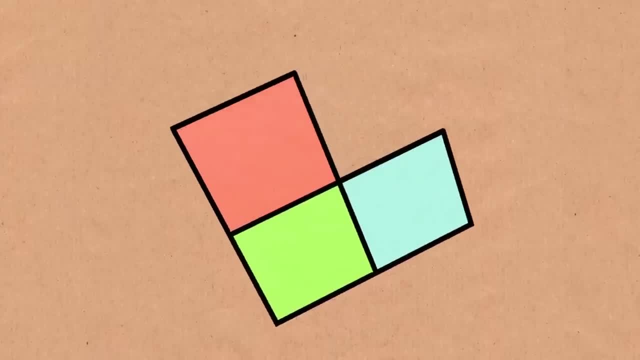 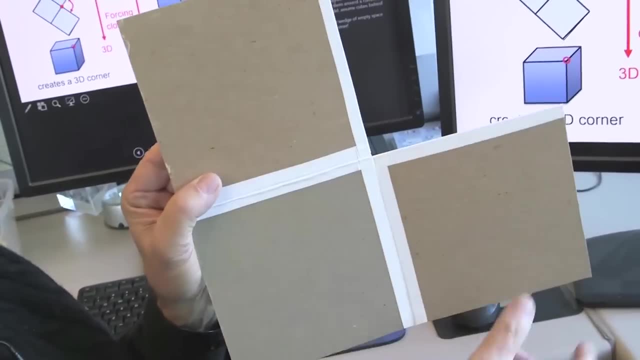 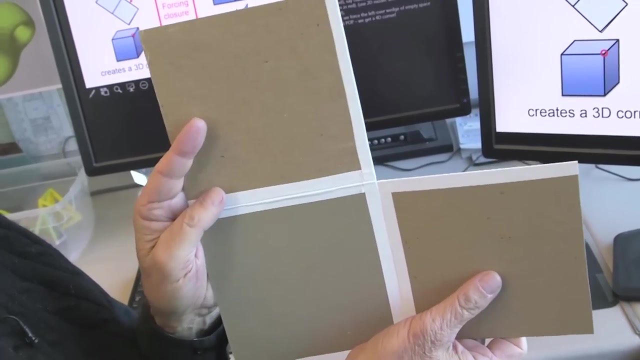 except think that behind each one of these squares there is a complete cube And these three cubes perpendicular to this plane in in that particular corner. So there's a 90-degree wedge of open space and we're trying to forcefully close that. And we cannot close that in three dimensions if there are. 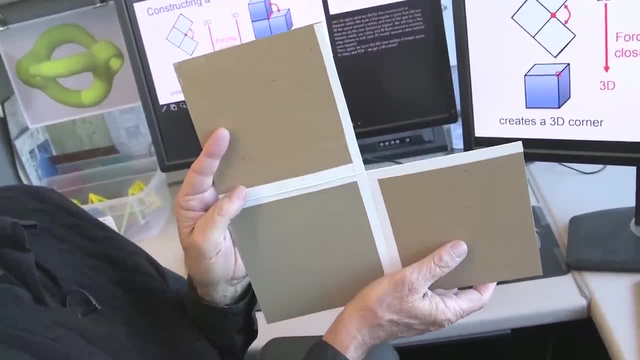 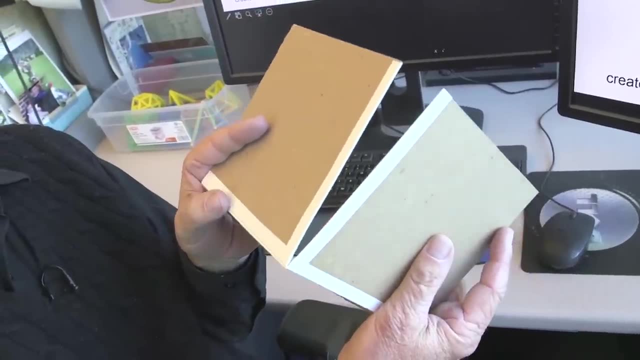 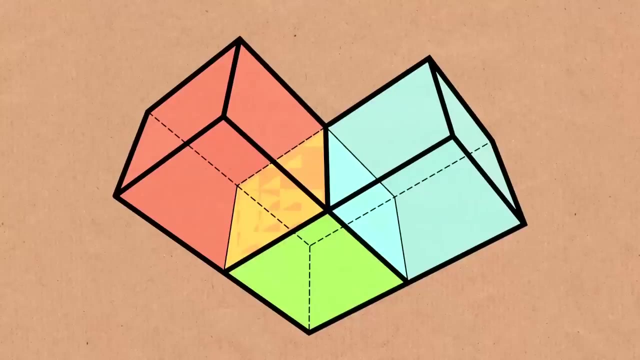 cubes behind each one of these four visible squares. But trust me, if we really do that and we can pop out in the fourth dimension, we can close up, you know, these cubes and we get a hypercube. Those cubes behind these that I was. 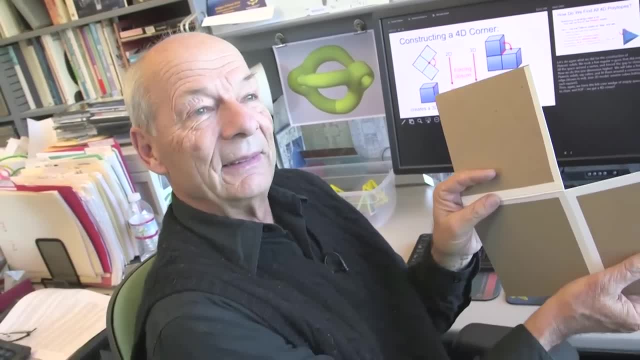 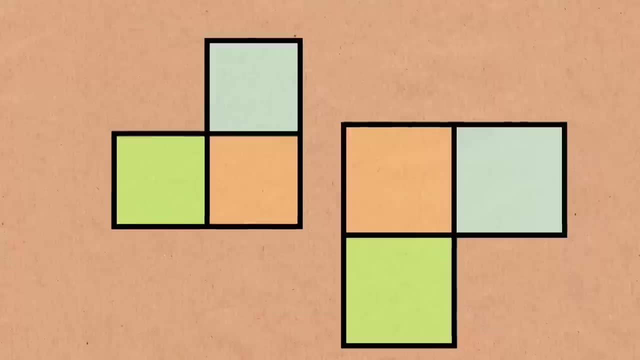 thinking about that. I've been asked to imagine they've kind of overlapped with each other. now No, because they pop out into four-dimensional space in the same way that when we took these two-dimensional squares and we forced them to close. they didn't overlap, They just popped out. 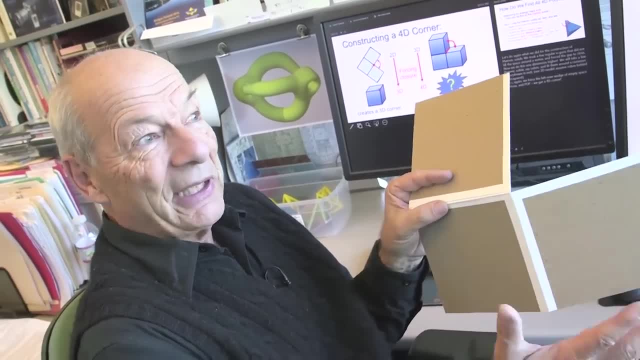 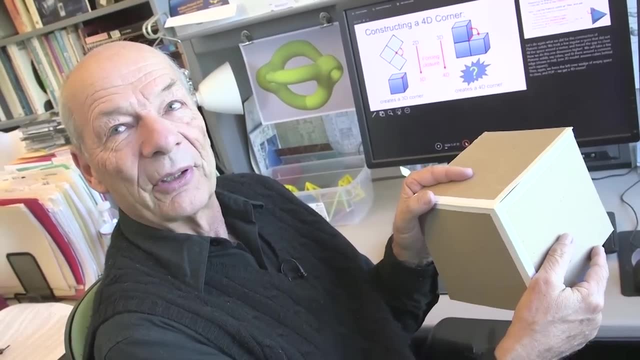 of two dimensions into three dimensions, And four-dimensional space is really much bigger than three-dimensional space, So there's ample room for these cubes to simply pop out and form a true four-dimensional corner. But to my three-dimensional eyes here sitting in 3D space, 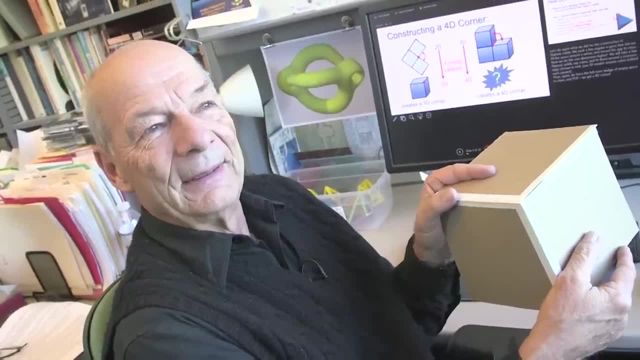 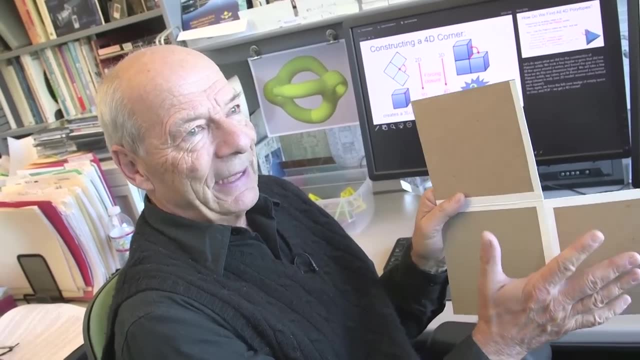 I'm like: how did that happen? But if I had four-dimensional eyes I'd be thinking That's correct. And now you're hitting on the real problem And so we can figure out that this must be possible. But then can we visualize that? I mean, how do you know what this thing looks like? 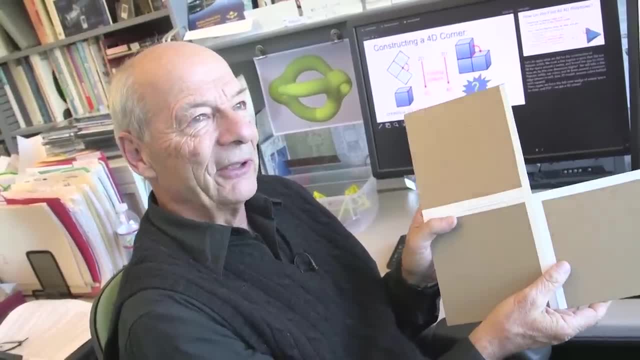 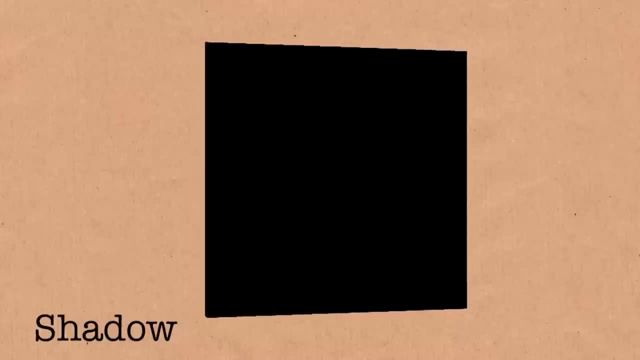 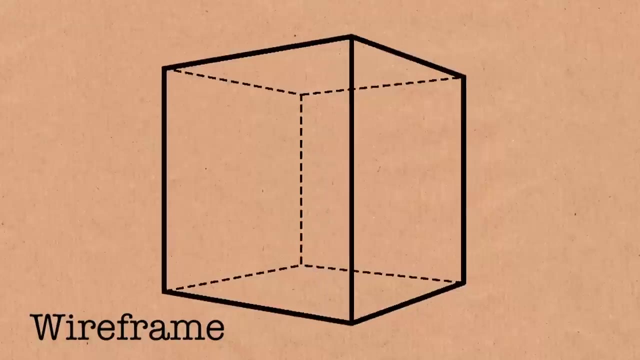 Well, for that we have to use some kind of a shadow or a projection of a four-dimensional object down into three-dimensional space. And I'm sort of torn between, you know, should we use a shadow or should we use What I would call a wireframe? And you see the trade-off between those two options. 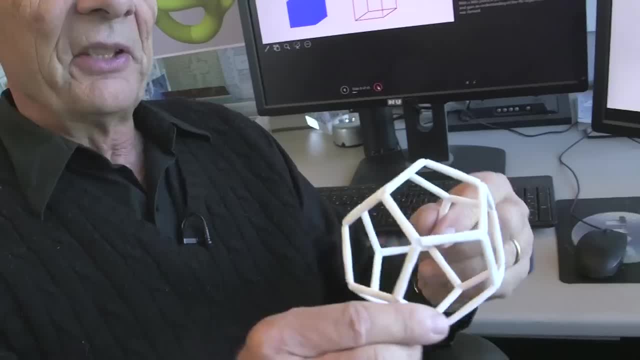 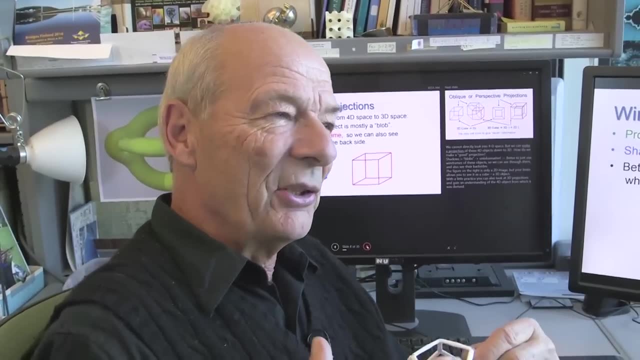 Just like if I show you the wireframe of the Dodecahedron. you can really see through it And it tells you much more than if you just had a faceless shadow of this object. You can eventually start to get a feeling by looking at three-dimensional wireframes. 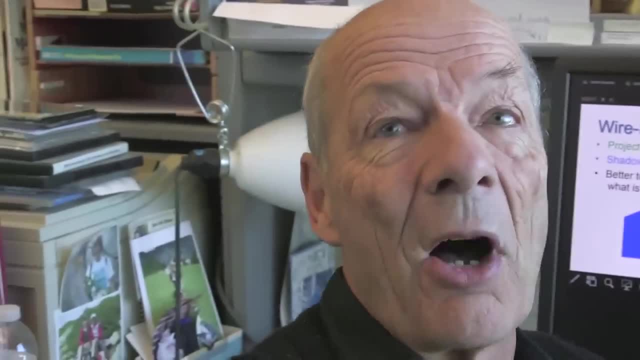 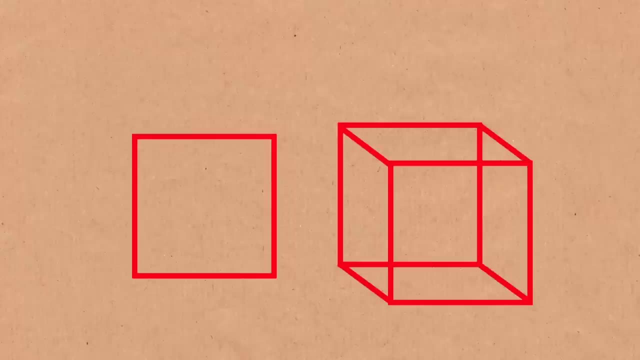 or projections of such wireframes, what the four-dimensional object might indeed look like. In doing this projection, we still have an option. We can project in various different ways. We're going from a two-dimensional square to a three-dimensional object And in an 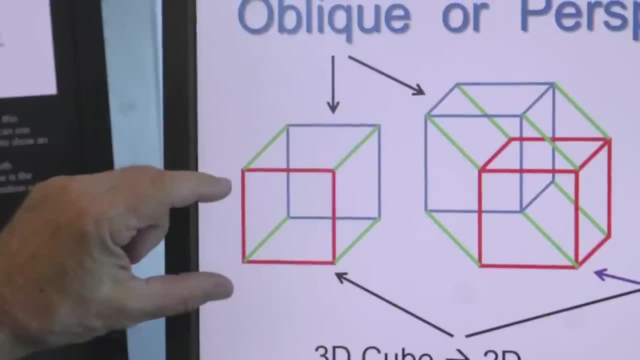 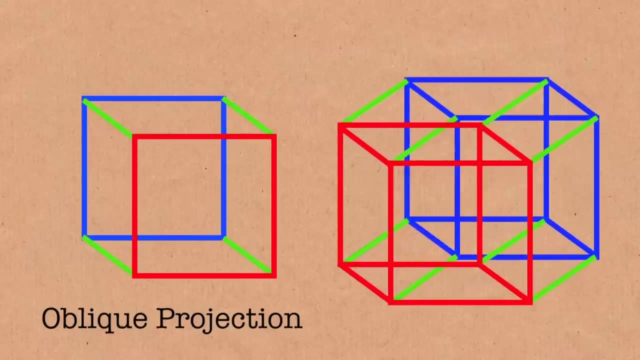 oblique projection. I start with the red square in front, and then the blue square is the ones in the back, and the green lines essentially show me the depth. We can do the same thing by starting with a complete cube: The red cube is in front, the blue cube is in the back and then 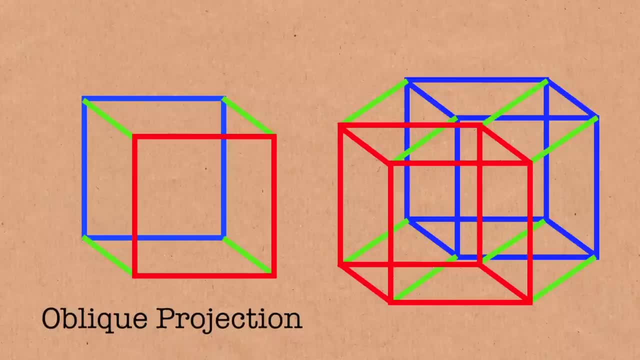 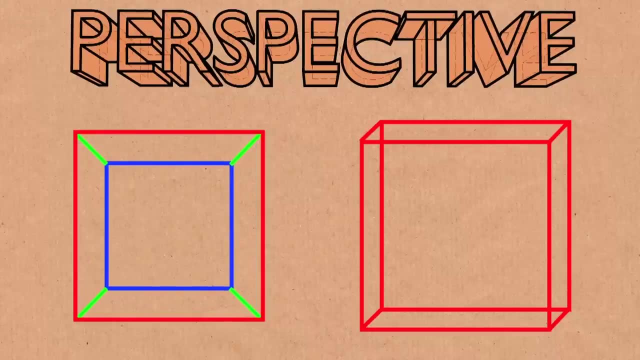 the green lines show essentially extrusion of this cube in this oblique direction. Alternatively, we can use a perspective projection. Everything in the back would appear smaller and we can look at the face And by doing that, you know, the back face will be a smaller square. so really behind, 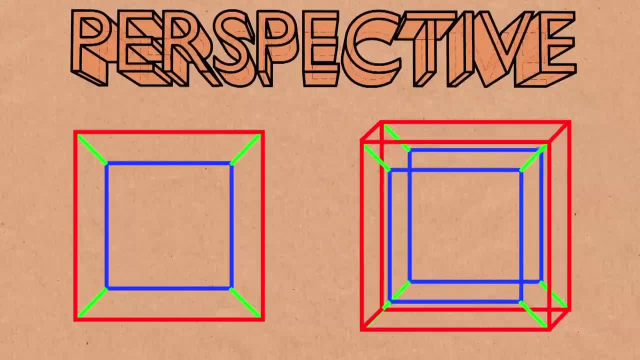 the red square and the green lines show kind of the depth going from the front to the back, And the same we can do with a complete cube and we get you know in the back a smaller cube shown in blue, and then the edges that go from the front to the back are shown in green. So here is the oblique. 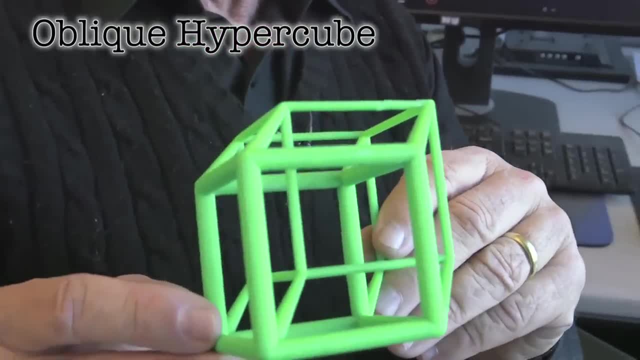 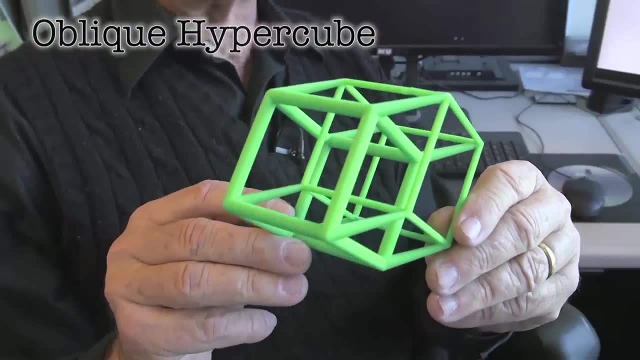 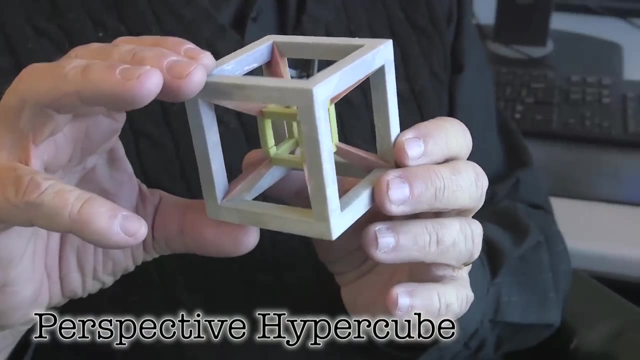 projection You can see the fatter cube being sort of the one in front and then the thinner cube in the back and then the slightly conical edges leading from the front to the back. So that's a valid depiction of a wireframe, of a hypercube. And here is the alternative model, a perspective projection. 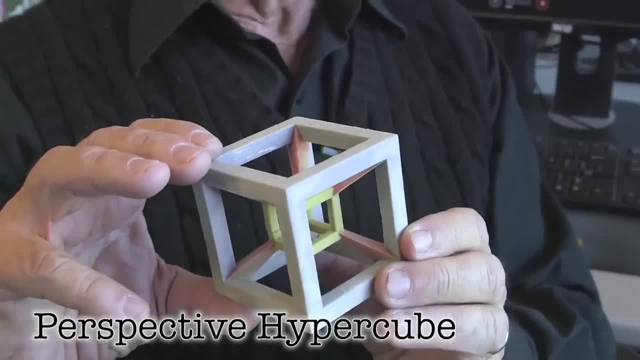 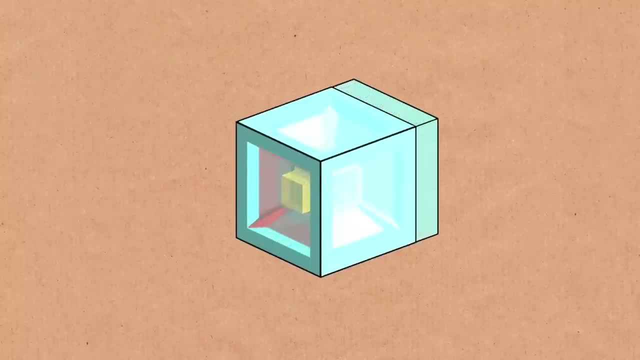 So the bluish cube is the front cube and the yellow cube is the one in the back, which is here much smaller, The red edges that go from the front to the back- And this hypercube has a total of eight cubes: The front cube in blue, the back cube in yellow and then some squashed cubes here. 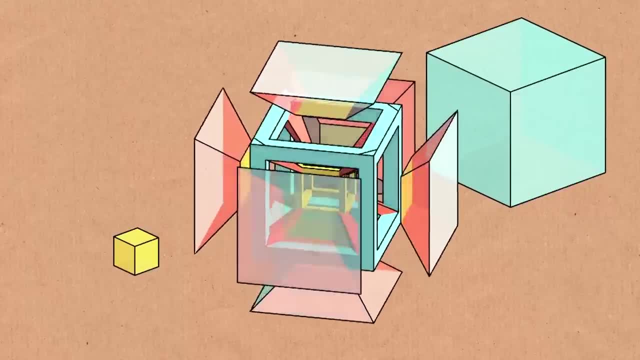 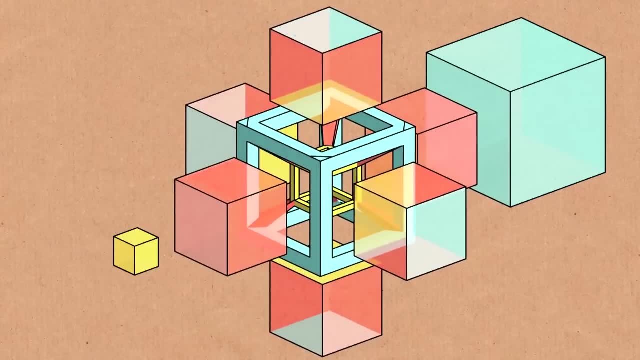 showing one on each of six faces. So there's a total of eight cubes making the surface or the thick crust of the hypercube. So that yellow cube isn't inside the blue cube. No, in four dimensions. it would be sort of up in the fourth dimension a certain distance. 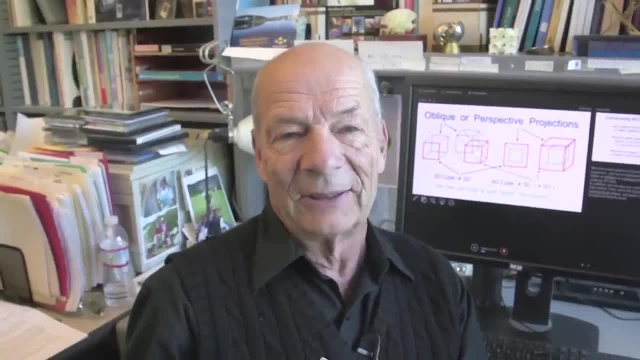 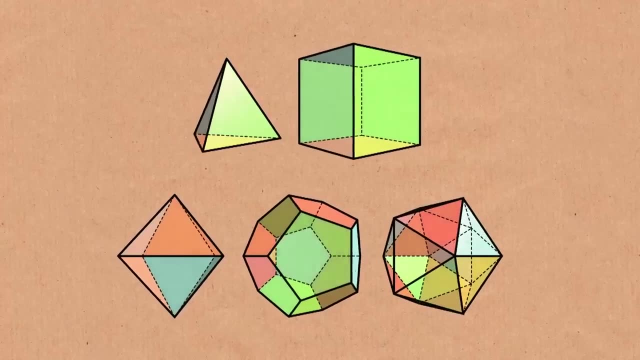 And because of perspective projection, what's further up there, you know, gets projected into the back and appears smaller in this projection. Now we're going to systematically look at all the platonic solids, see how many we can group around the shared edge, how much empty space there is. 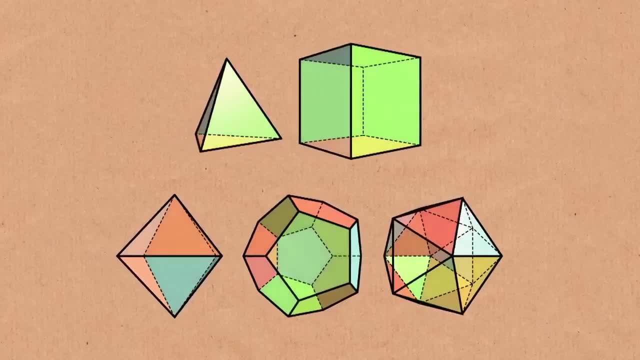 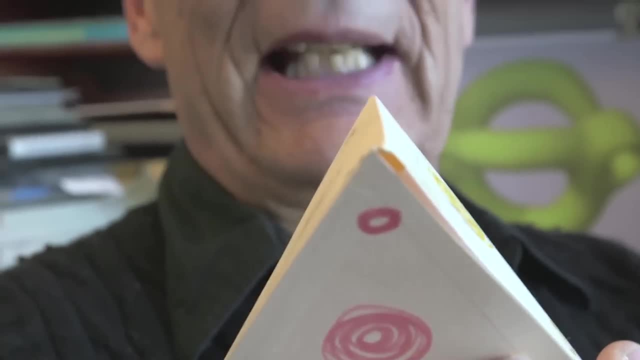 and then we push that one out and push that into a valid 4D corner. The simplest object to start with is the tetrahedron. The tetrahedron has a dihedral angle of 70 and a half degrees. We need at least three of these tetrahedrons around the edge to make a valid corner Three. 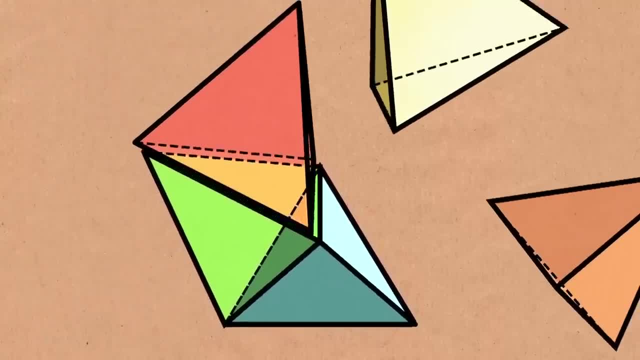 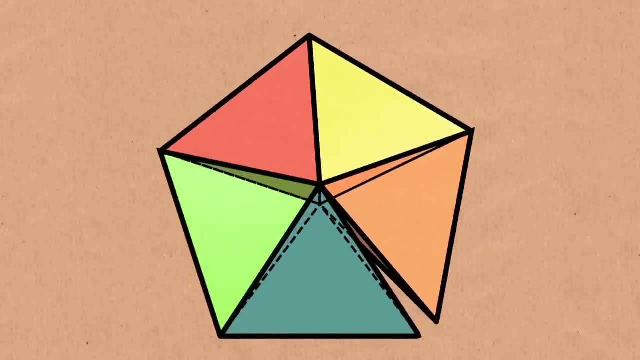 of course, fits very easily: Four fits, Even five fits, but just barely. We just have a few degrees left, And so when we try to fit five tetrahedron around this, we just get a little bit bending in four-dimensional space And we will need, as we will see, a whole lot of these tetrahedra to make. 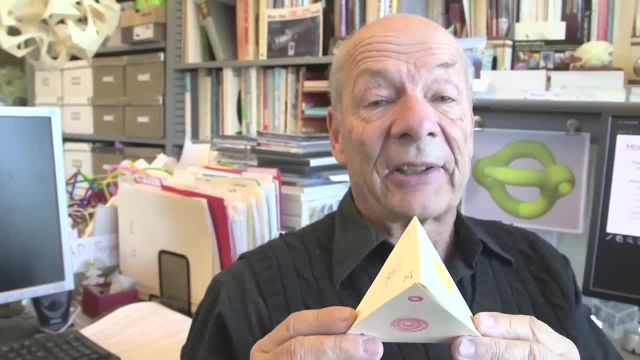 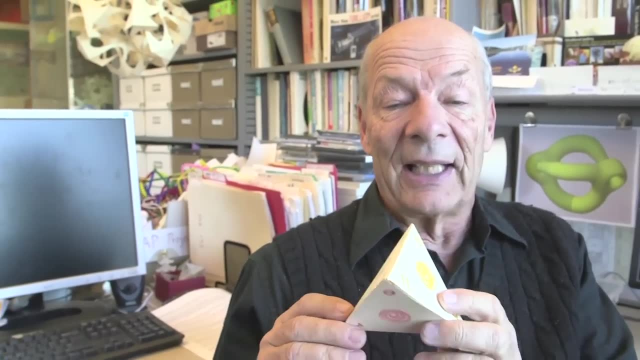 it actually work out. So we can start out with three tetrahedrons and ask what happens if we forcefully, you know, bend that into a corner? Can we repeat it? And the answer is we will get the simplex or the five cell. So because of the projection, 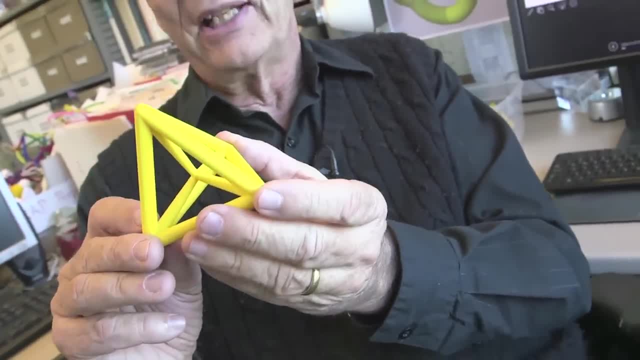 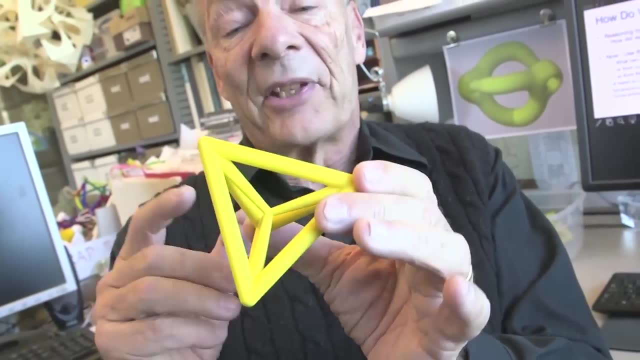 you know, it becomes just a three-dimensional object and it loses some of its symmetry. So we have five vertices, but the fifth one, to make it as symmetrical as possible, I put here right in the middle. So we get the outer tetrahedron and then we get the dimples here. 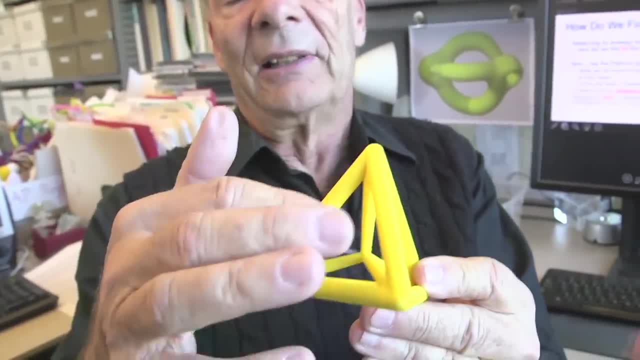 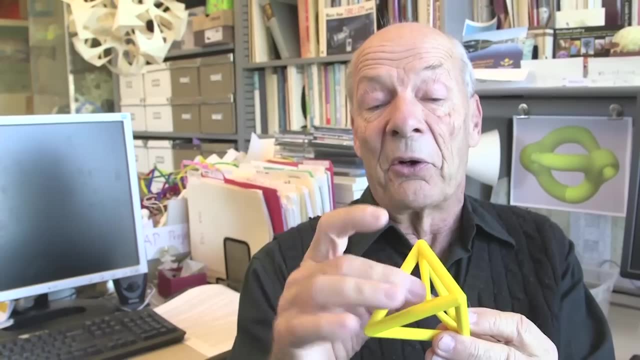 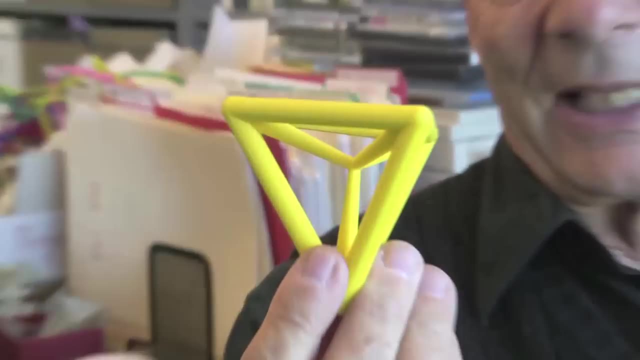 on each side. They all represent additional four tetrahedra and they don't look very regular, And that's because of the projection. but in four-dimensional space all five of these tetrahedra are completely irregular, and so that's the five cell or the simplex. That's what happens. 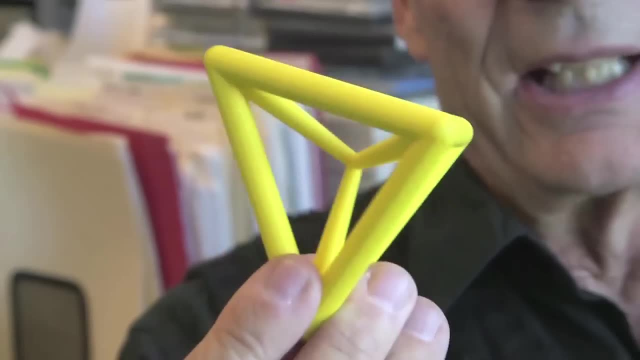 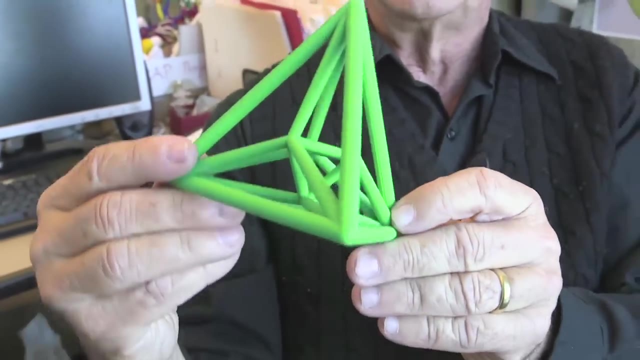 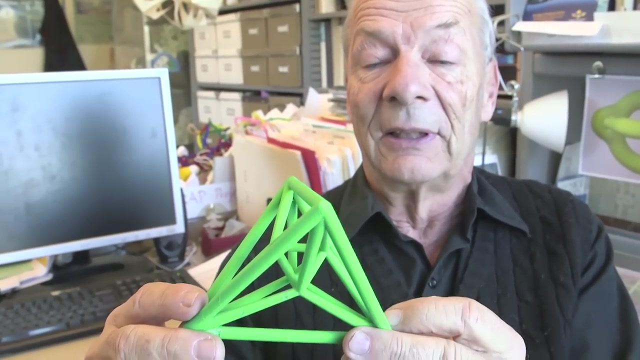 when you take three tetrahedra around the shared edge and essentially force out the empty space and bend them into a true four-dimensional corner, Four tetrahedra around the corner, you know we get this object here. Okay, it's called the cross polytope and it's actually the dual of the hypercube that we've seen before. okay, 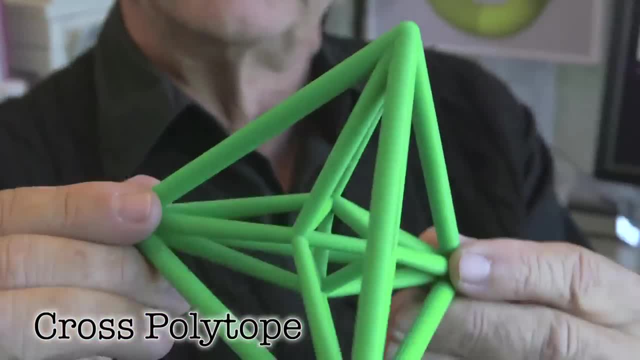 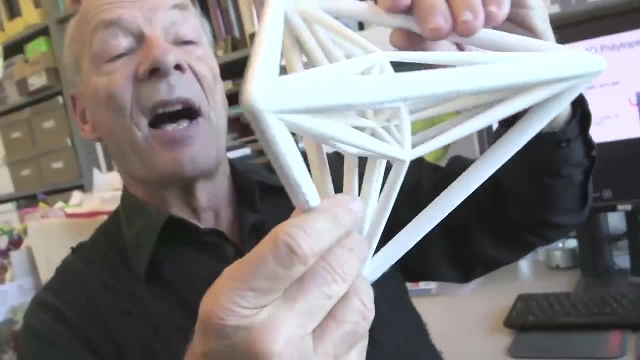 So that's the cross polytope, the second regular polytope in four dimensions, Five tetrahedra. put it around the sheared edge, you get something that has a lot of tetrahedra. As a matter of fact, this thing has 600 tetrahedra. 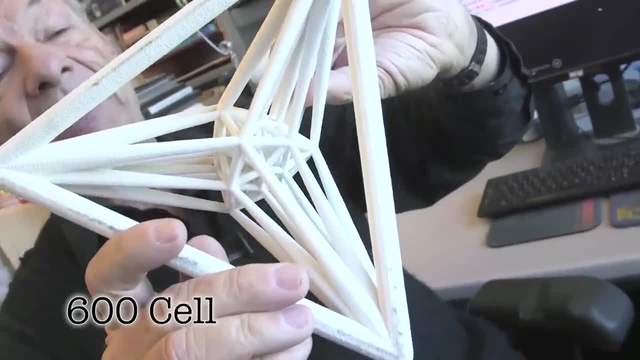 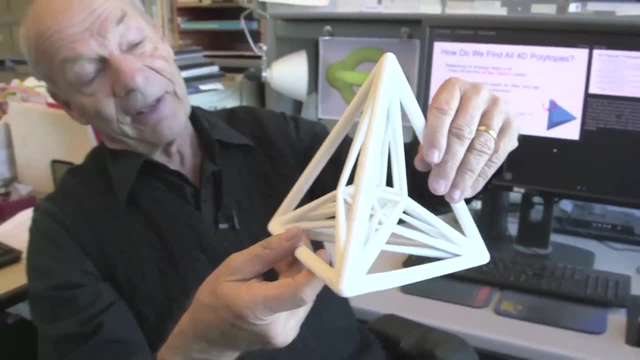 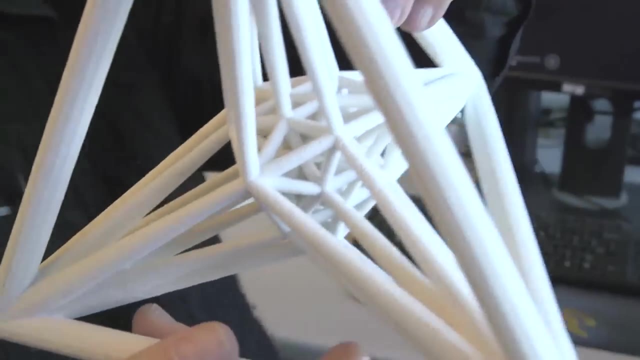 Most of them are sort of crunched up in the middle here because of the projection, and you just see one giant tetrahedra on the outside and then, adjacent to each faces, you see smaller, fairly much flattened out tetrahedra, and you have to just believe me that in there 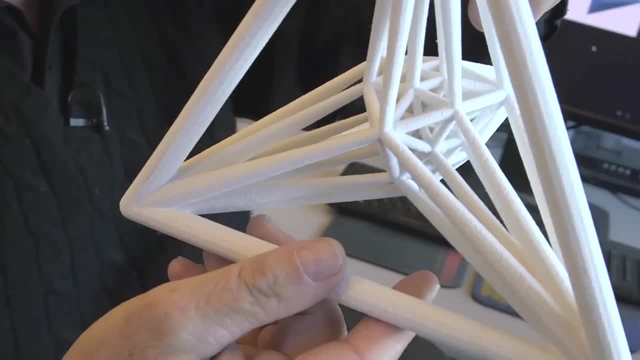 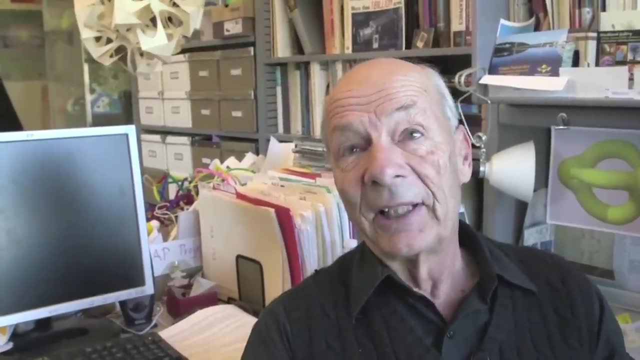 there are essentially, in addition to this one out here, another 599 tetrahedra. This is called the 600 cell. Six tetrahedra would exceed the dihedral angle of 360 degrees and that's, like you know, something warped. that is not regular. 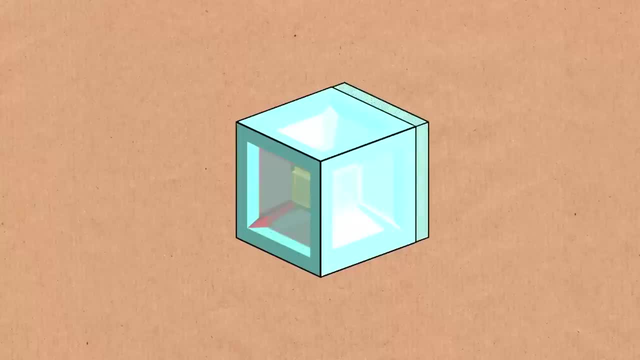 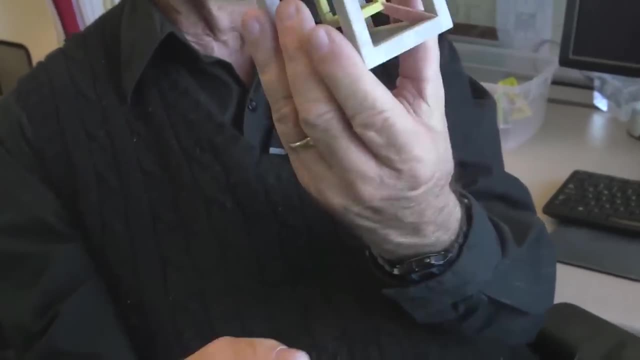 so that's of no use. We have seen cubes. They have tetrahedral angles of 90 degrees. Three of them will fit around an axis, still leave an open gap, and then we fold this one up. we've seen: we get the hypercube. 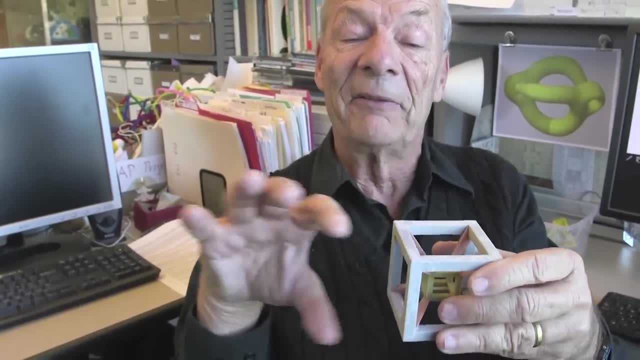 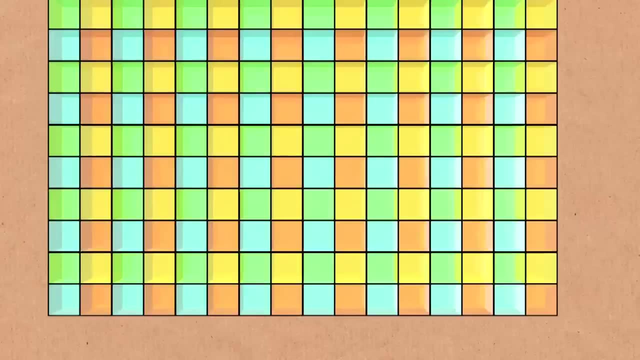 If you try to put four cubes around the joint axis, you can readily visualize that would readily fill the space without any bending, and so you can tile all of three-dimensional space with that. but it will never bend and make a regular polytopes in a higher dimension. 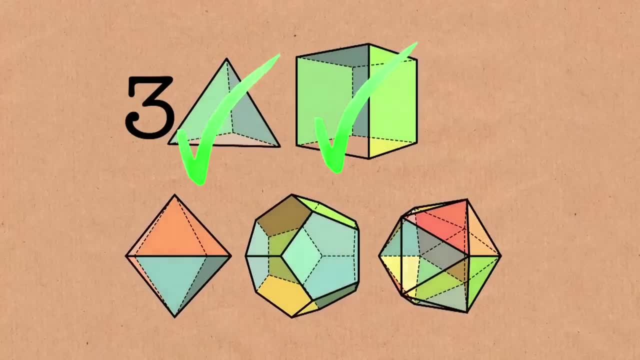 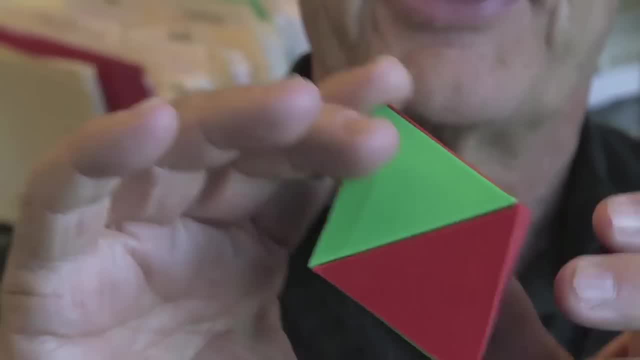 So we're done with the cubes. The next platonic solids we may want to try is the octahedron. It has a dihedral angle of 109.5 degrees, so that's less than 120 degrees here, and that means we can indeed fit three around a joint edge. 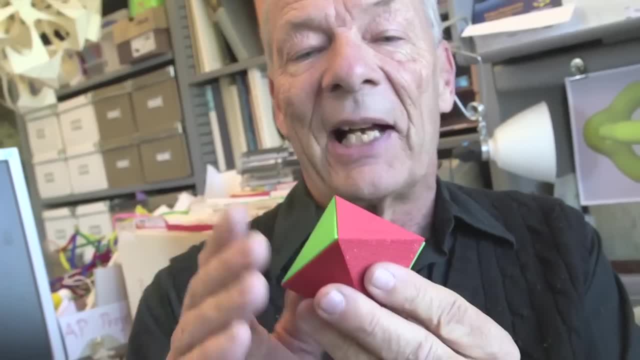 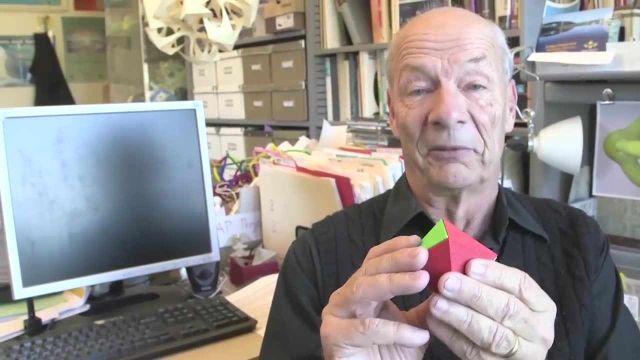 and still leave a little bit of open space which we can squeeze out and make. this then pop into the fourth dimension And the result is what I believe to be the most beautiful four-dimensional regular polytope: the 24 cell made up of 24 octahedra. 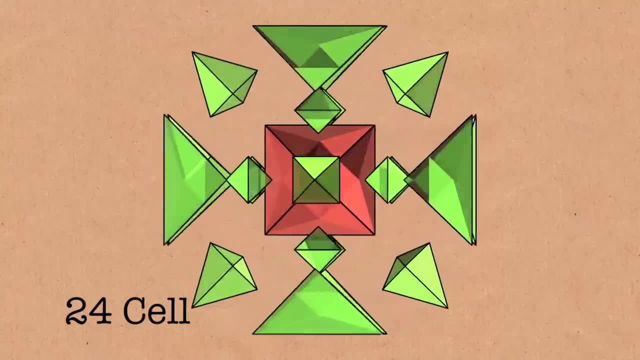 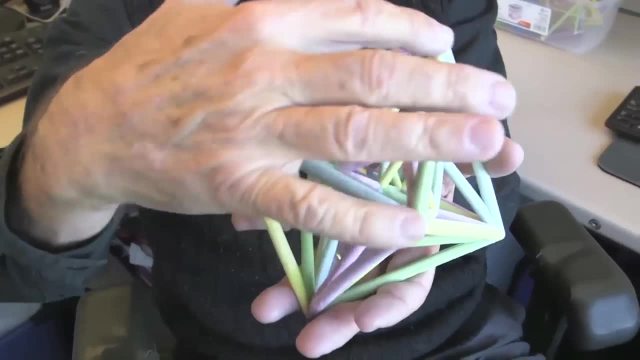 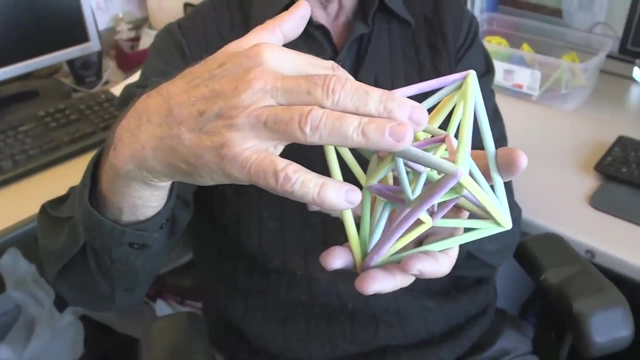 You can see the outermost octahedron, because I chose that to be, you know, preserved in the projection. but then you see these rather flattened octahedra, with one triangle here, another triangle, the small one here, and sort of a distorted antiprism in between. 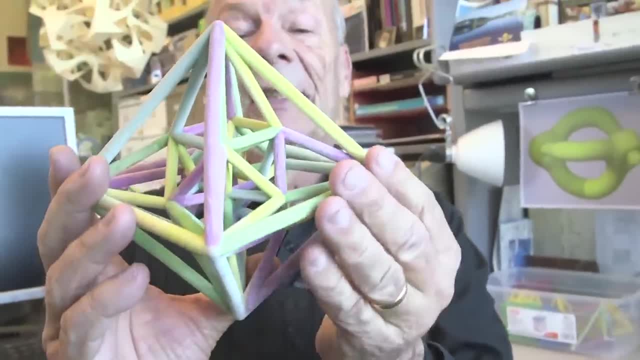 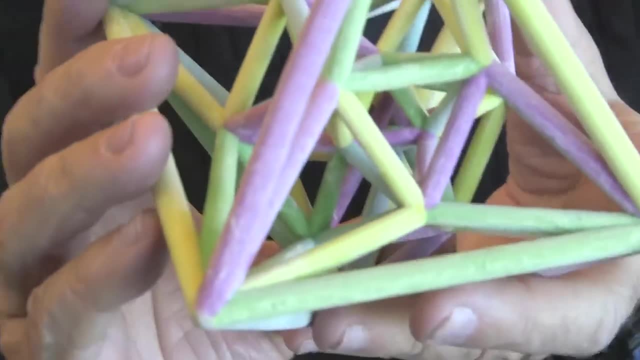 and then they're more on the inside. I really like this particular object the most because it's not too complex. You can still see what's going on. You can still look on the inside and see the innermost, very tiny little octahedron at the center. 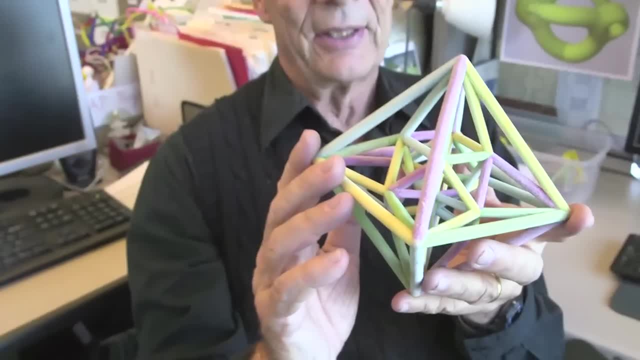 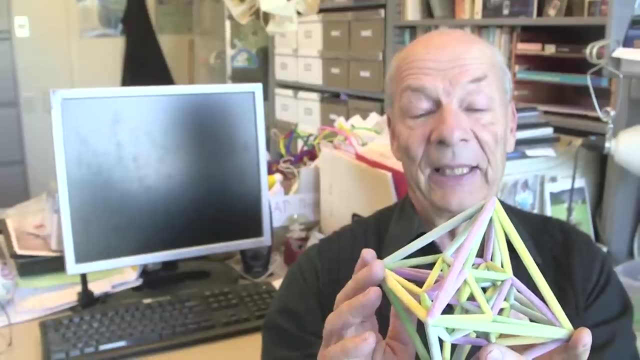 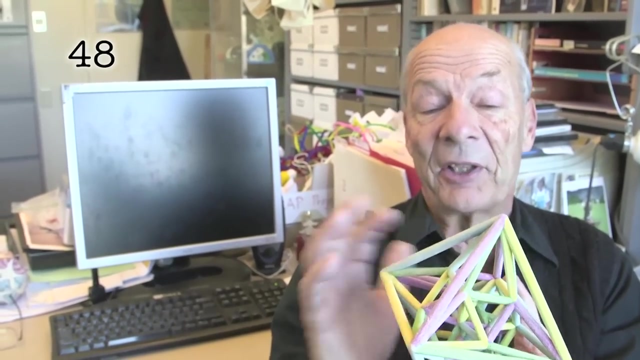 Now it turns out that the octahedron is a little bit smaller than the other octahedron. It turns out this object has 1,152 symmetries in four-dimensional space, And you simply get that by multiplying the symmetries of an octahedron, which are 48,. 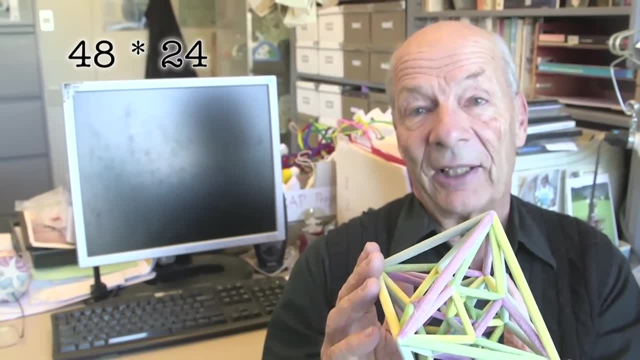 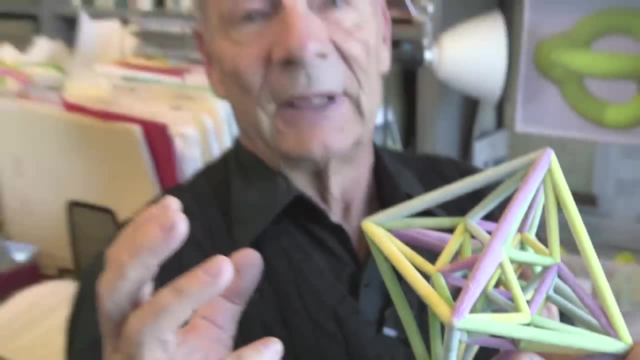 with the number of octahedra 24.. You multiply this out, you get the 1,152, because you can take in four-dimensional space any one of the octahedron by a suitable rotation of any one of the other 24 octahedra. 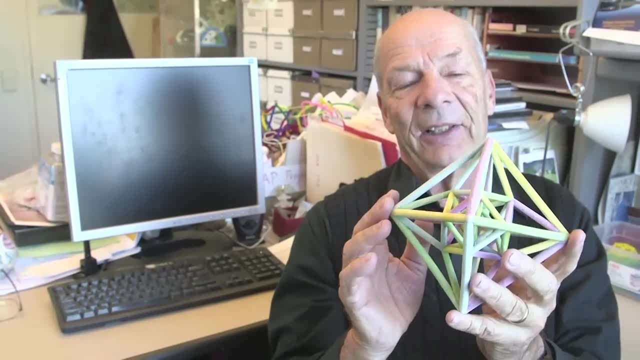 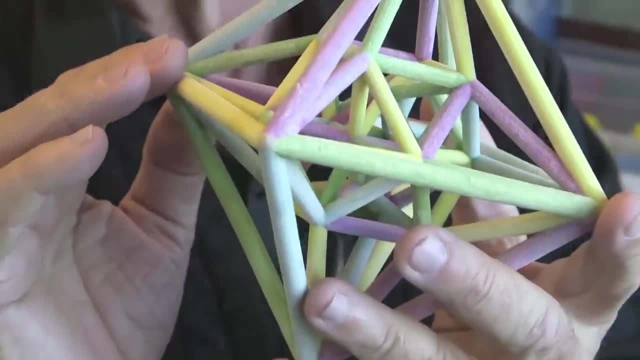 in any one of the 48 possible positions. I live at the street address 1,152.. And when I found out that this object has 1,152 symmetries, I thought that somehow fate really meant me to be, you know, into geometry. 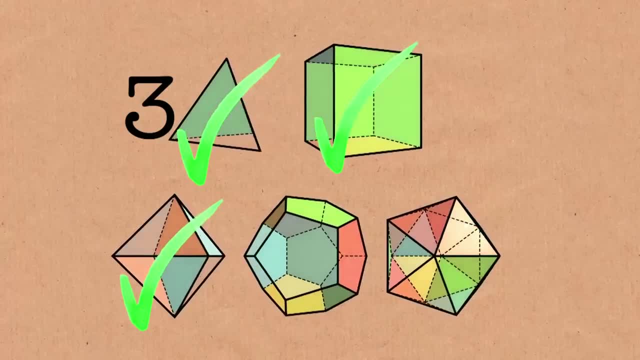 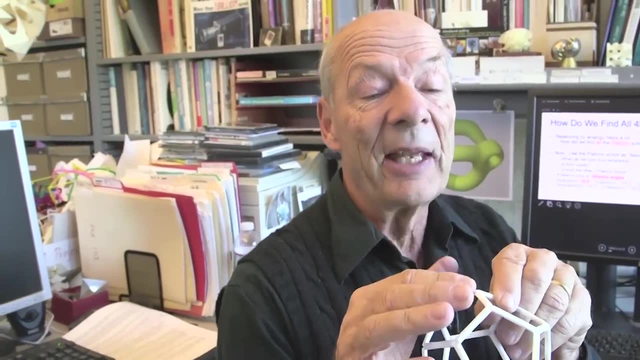 The next one on the list is the dodecahedron. It's 116.5 degrees of a dihedral angle. That is still less than 120 degrees, so we can still force it, Force three of them around an edge. and then join them into a valid four-dimensional corner. It's not bending all that much, and so we will need 120 of those objects in the crust to form a valid four-dimensional regular polytope. So this is a model of the 120 cell. 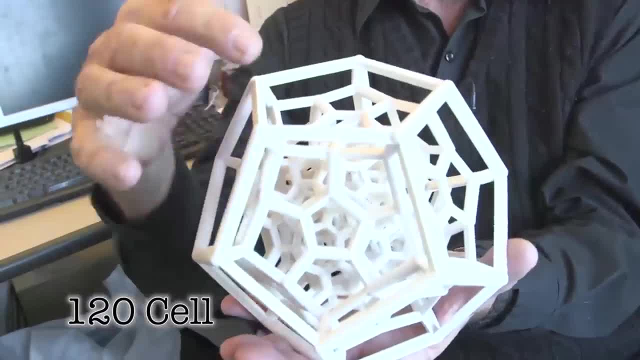 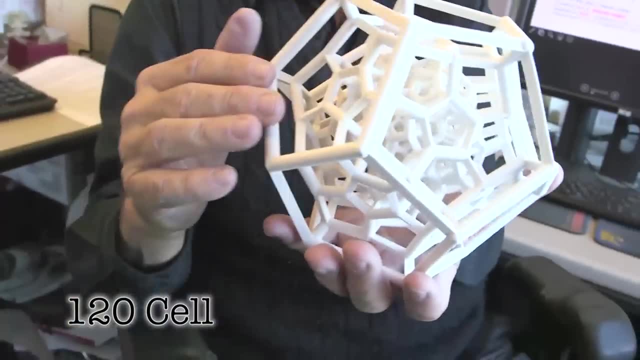 Of course you can see the outermost dodecahedron. You can also see kind of this flattened pancake-like you know dodecahedron top here And each one of the faces has one of those, and then stacked on the inside there are a few more added. 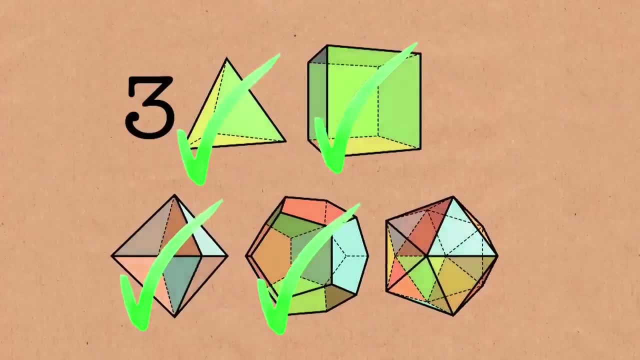 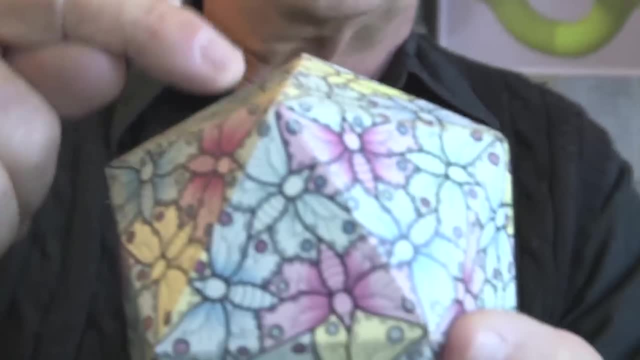 Adding up to a total of 120 of those. We still have the icosahedron. Unfortunately, it has a very shallow dihedral angle. It is more than 120 degrees. It is actually 138 degrees roughly, And so even three of them would not fit around this edge without overlapping. 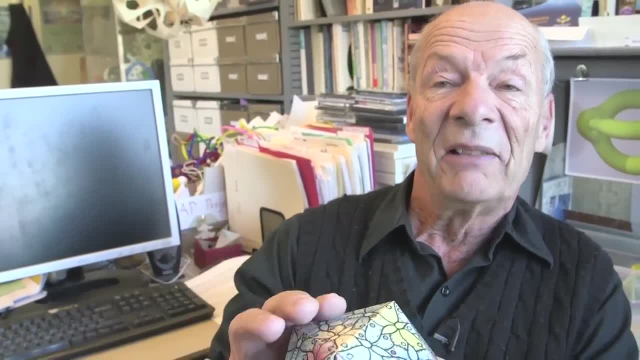 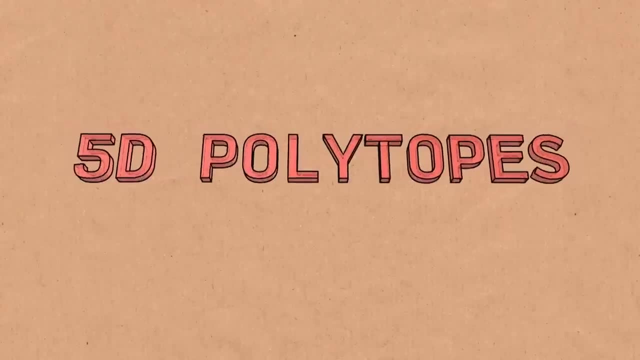 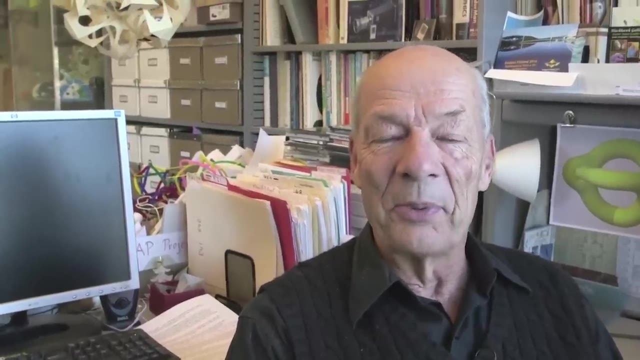 and so we cannot form a valid corner And unfortunately, this is useless. as far as making a four-dimensional regular polytope, You basically can figure it out yourself. right, You know how to make five-dimensional regular polytopes. You look at the four-dimensional regular polytopes. 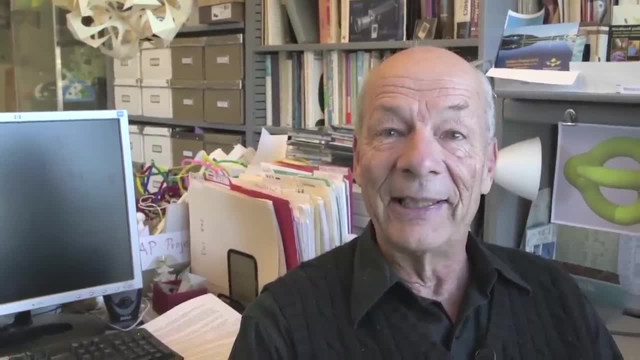 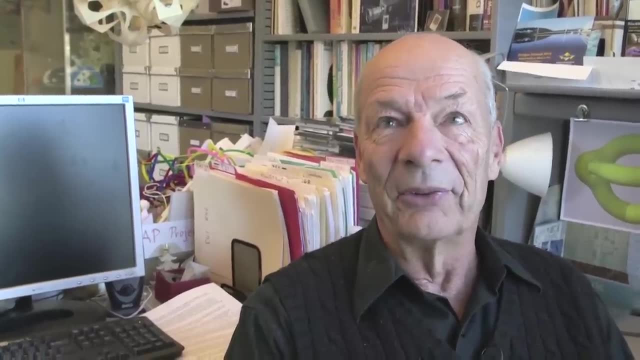 look at their dihedral angles and figure out. you know, can I fit at least three of them around an edge so I can make a valid corner. Most of these regular polytopes in four dimensions are very round and they are not very useful. 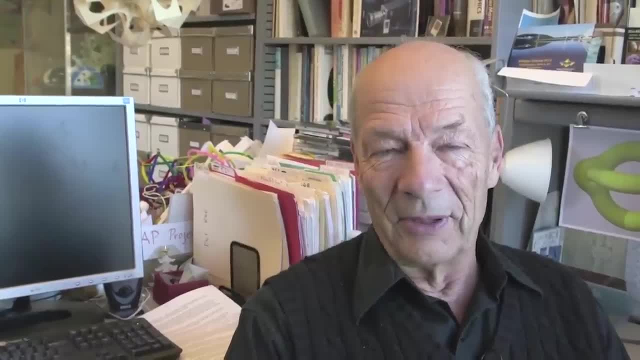 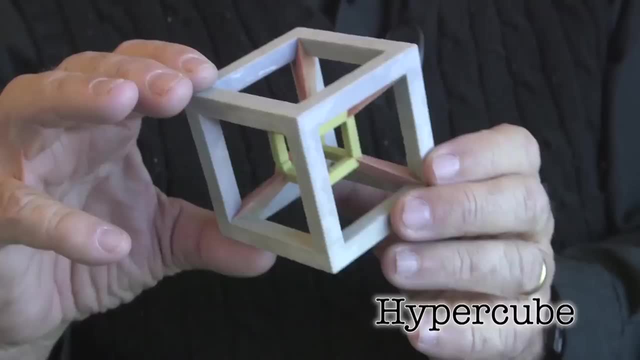 There are really only two of them that actually have some hope of generating a new regular polytope in a higher dimension. One of them is the simplex, or the five cell, and the other one is the hypercube. The other ones have got two shallower angles. Yeah, the other one have two shallows of dihedral angles and they just don't make valid corners in the next higher dimension. And so from five dimensions onwards, there are really only just three regular polytopes in each one of these dimensions. 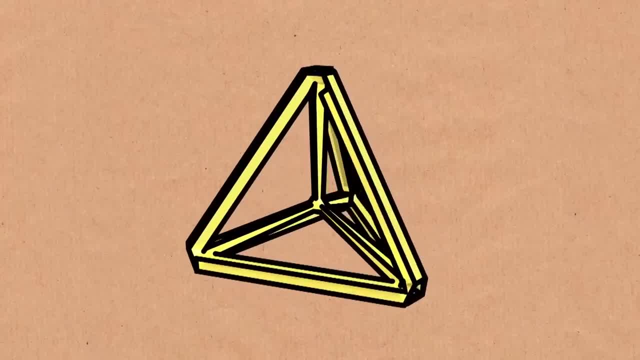 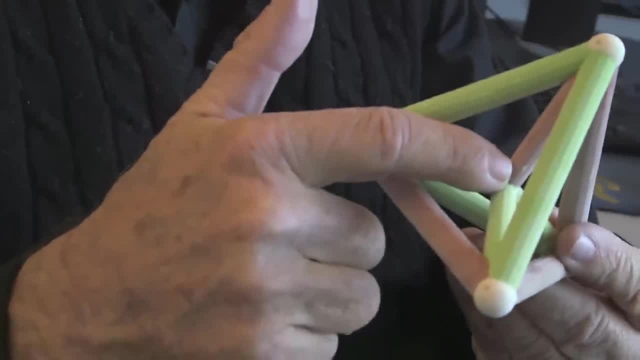 One is the simplex series. You can always make a simplex By taking a simplex in a particular dimension. I'm starting with the tetrahedron, and then I put another vertex at the center of gravity, And now I use the fourth dimension. 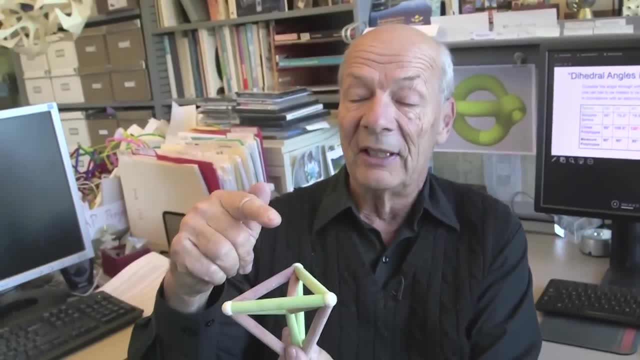 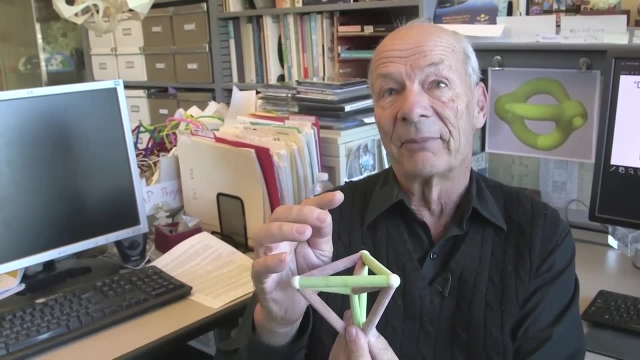 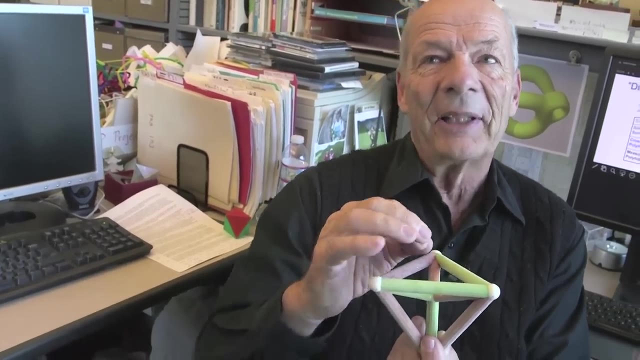 and essentially raise this vertex up in the fourth dimension until it has exactly the same distance from all the other four vertices. That makes a new simplex. And then I can take that particular simplex: put the new vertex at its center, raise it up in the next higher dimension. 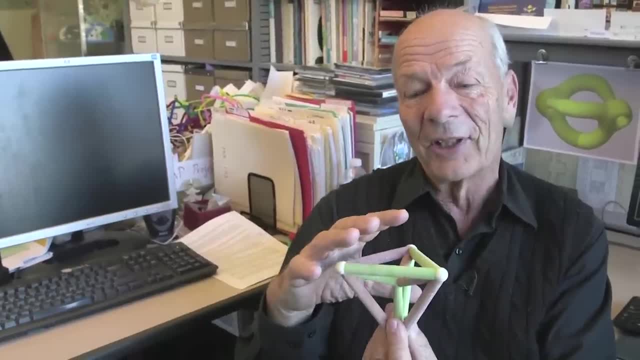 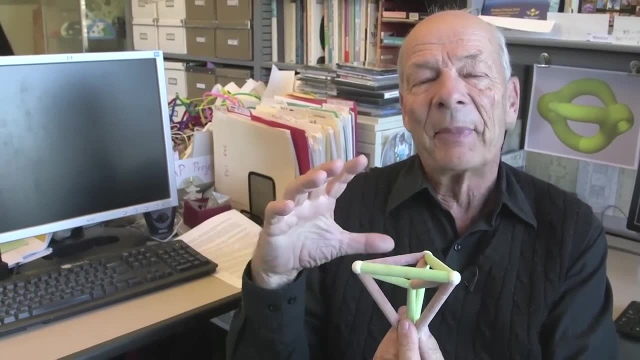 until it is exactly the same distance from all the previously existing vertices and make the next simplex. That always works, So I can work my way up to infinity by always making an additional simplex in exactly that manner. The problem now is: how do we depict those things? 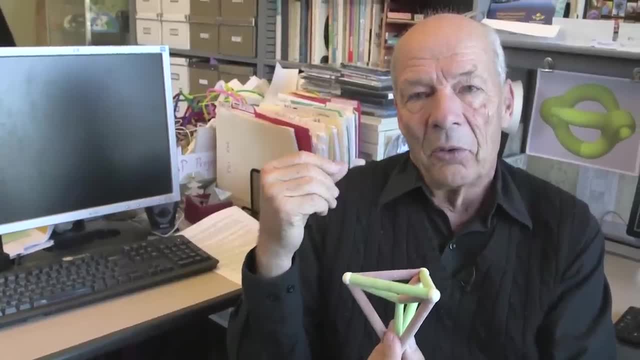 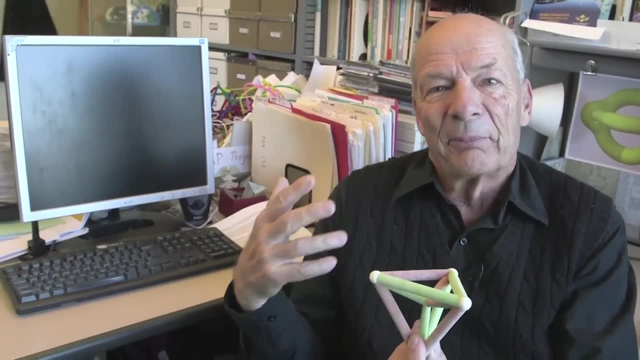 Because clearly, projecting it down, it could do anything. So it's better to figure out how do we make a model that has the right connectivity, even though the geometry really is sort of bogus at this point because it's so much distorted from what we originally have. 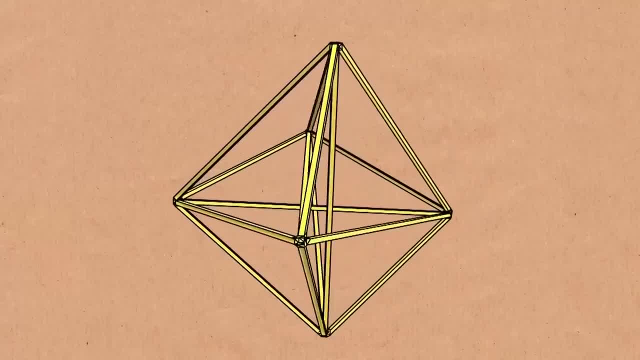 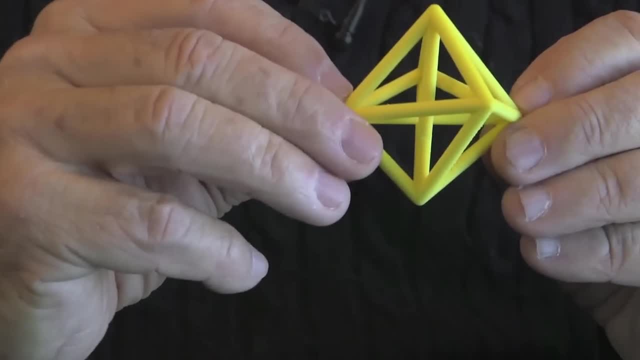 And I have made a few more simplices in higher dimensions. You just need to always add one more vertex and then figure out how to make a nice little graph that will get the right connectivity. So this one has six vertices. I claim this is a projection of the 5D simplex. 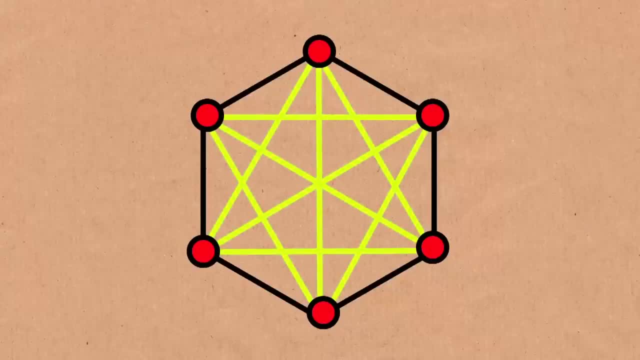 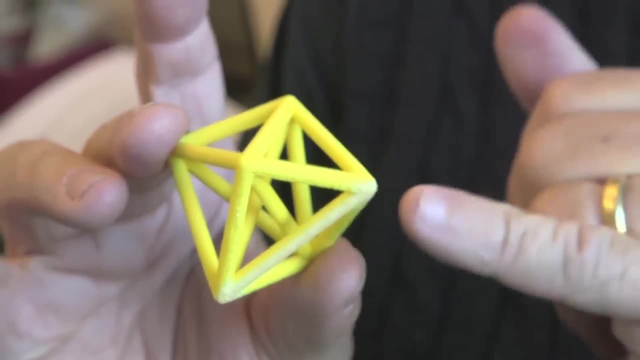 because the simplex also is the complete graph. Every vertex is connected directly to every other vertex And you can see- in this case you start at any one vertex- there are five edges going off one to each of the other vertices, So we want to make a 3D model that has six corners. 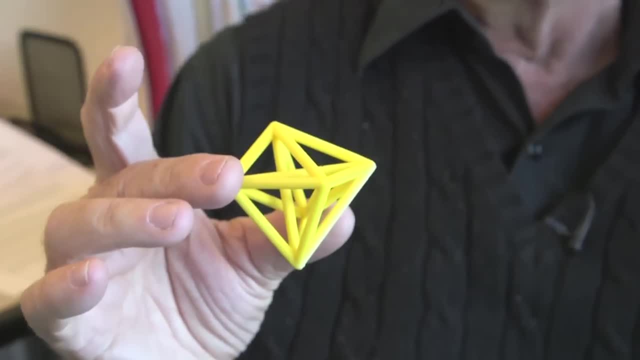 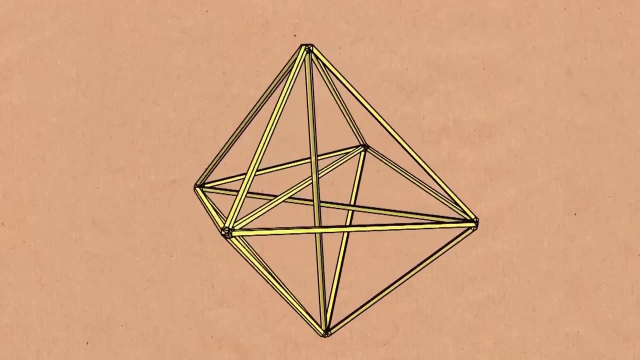 is reasonably symmetric, but not too symmetric. So we could start with an octahedron, but in the octahedron then when you connect opposite vertices, those three edges will all intersect in the middle. That wouldn't be so nice. you wouldn't see what's going on. 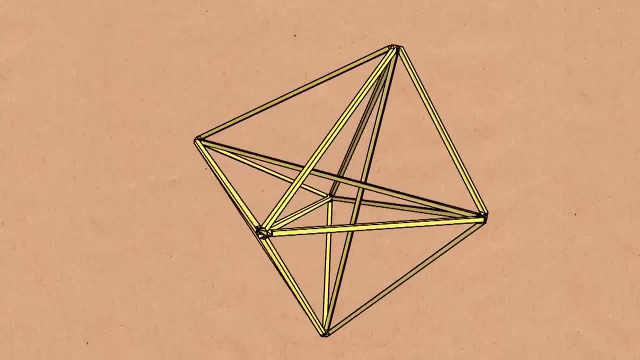 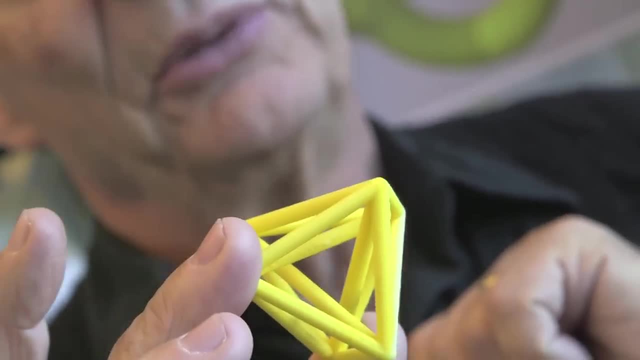 So I had to deliberately distort this octahedron, warp it a little bit so that those three space diagonals that go through the middle of the regular octahedron they have separated out and now they do not intersect with each other anymore. 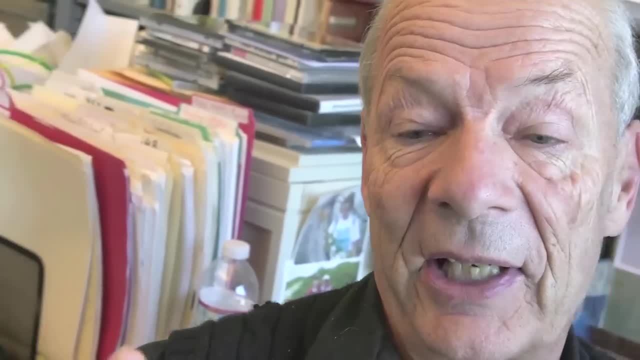 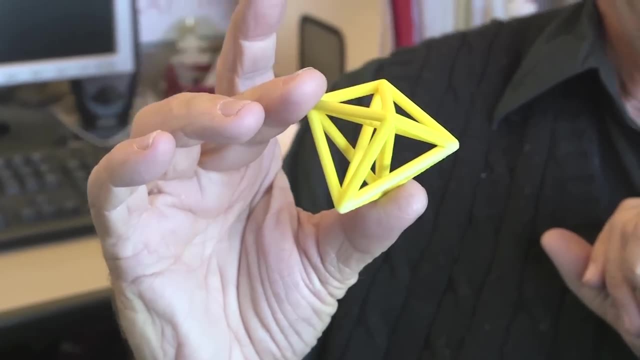 So the trick was really just finding six vertices in a relatively symmetrical arrangement so we can connect every one with every other one without any intersections, And that's the game that we have to play for every one of the dimensions that we want to build a simplex model. 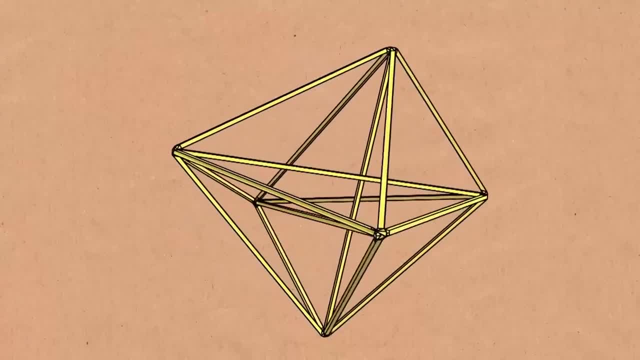 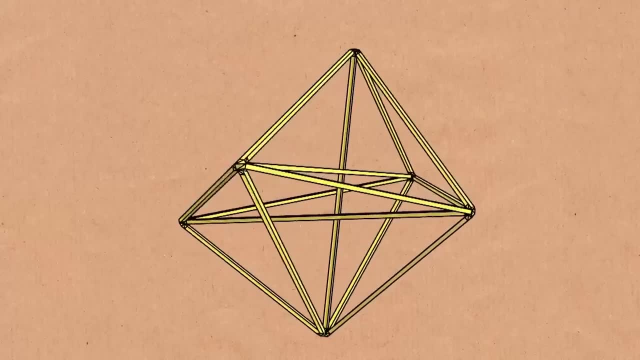 We already had this object that had six vertices, completely connected- the warped octahedron- and that actually has an extra free space in the center. It's easy, therefore, to put a seventh vertex right here in the center. This one can again be connected to all the other vertices. 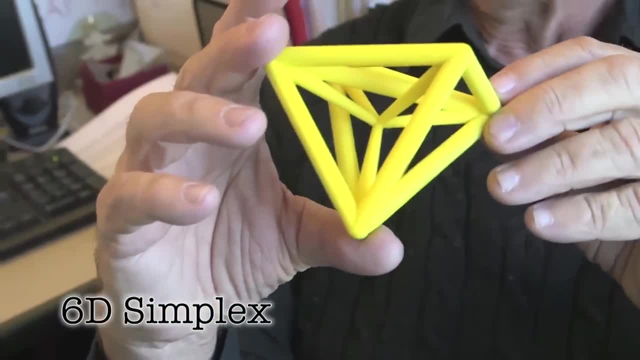 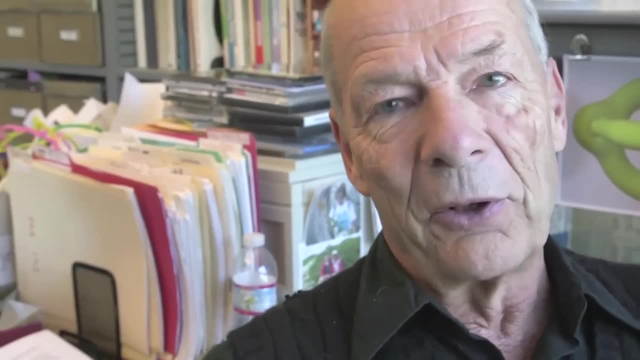 And so now we have a complete graph of seven vertices, and that would be a nice model of a six-dimensional object. This is a three-dimensional simplex. There is a second sequence that works for all dimensions, and it's called the measure polytope or hypercube sequence. 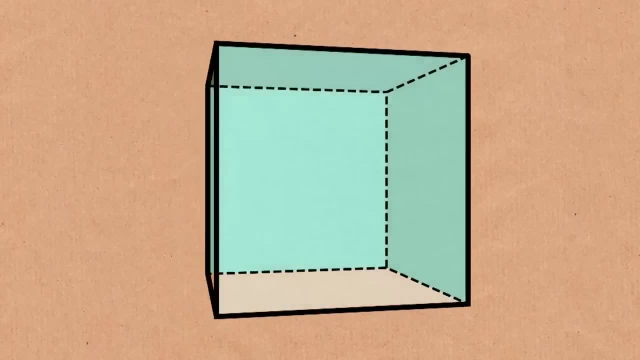 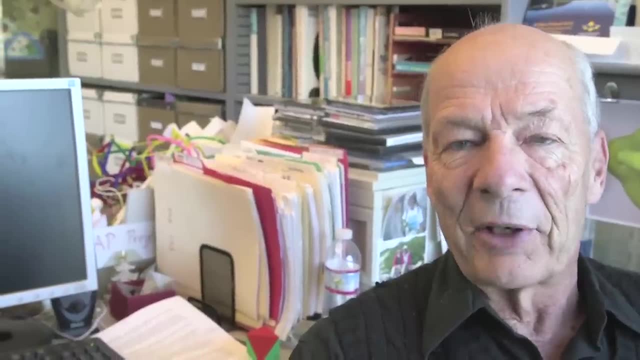 The cube is the object with which we measure the volume of three-dimensional space, just like the square is the geometric element that we use to measure two-dimensional space. Similarly, the hypercube would measure four-dimensional space, so the measure polytopes are always the equivalent. 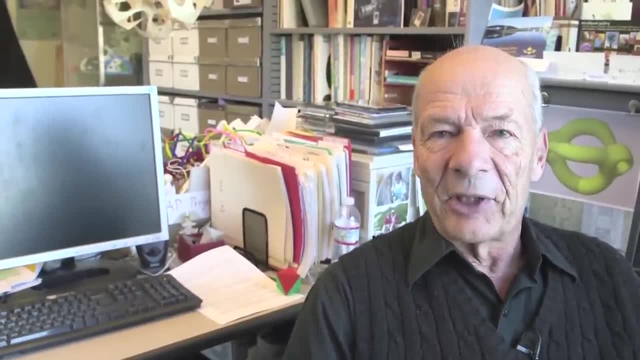 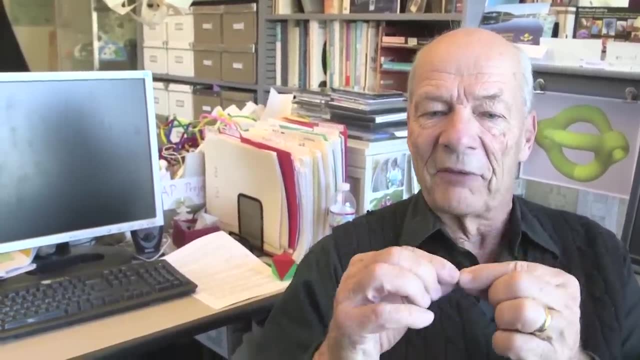 of a cube in the higher dimensions, And the best way of visualizing what's going on is essentially going in stepwise in extrusions. So we start with a line and then we take this line and extrude it basically into a square. 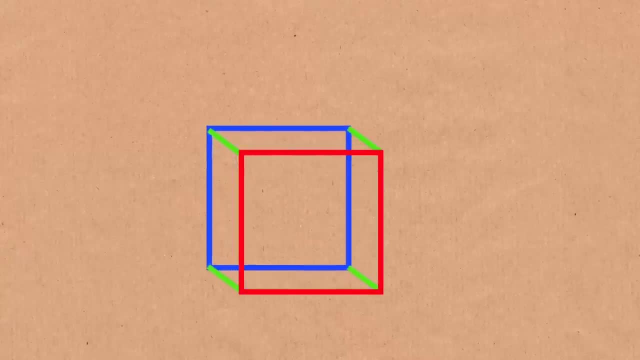 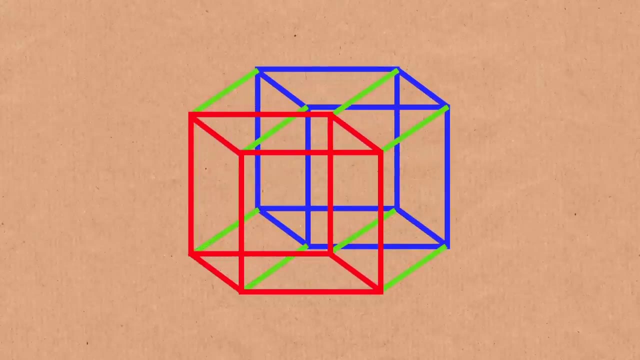 and then we sort of take that square and extrude it perpendicular to itself into a cube, and then we're doing one more extrusion of that cube into a hypercube. do an extrusion of the hypercube into the 5D measure, polytope? 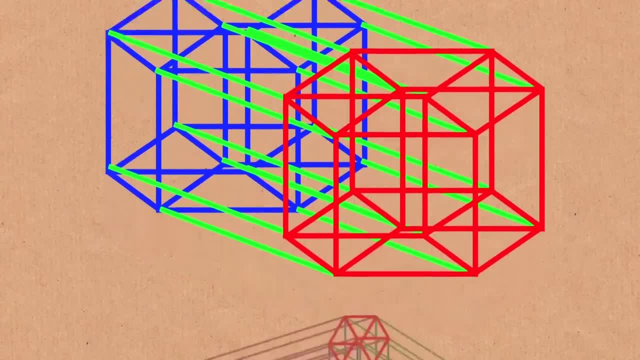 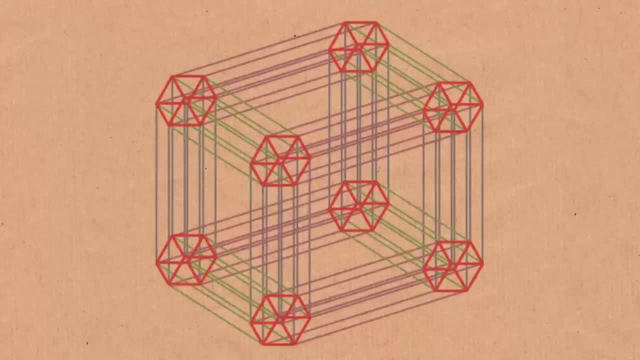 and you could continue that way or you can change the scale. So what I prefer, maybe in six dimensions, would be to take a regular cube and essentially sweep it in three different dimensions to make sort of a thickened cube frame which is showing every edge. 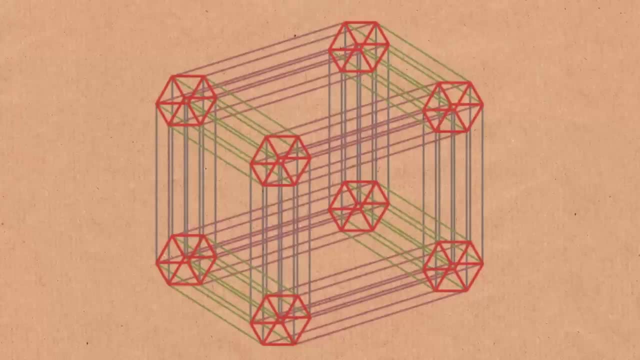 as the sweep path of one of those cubes. So this particular diagram would be a depiction of a six-dimensional hypercube which you get by extrusion. Another projection of the six-dimensional hypercube results in this rhombic triacontahedron. 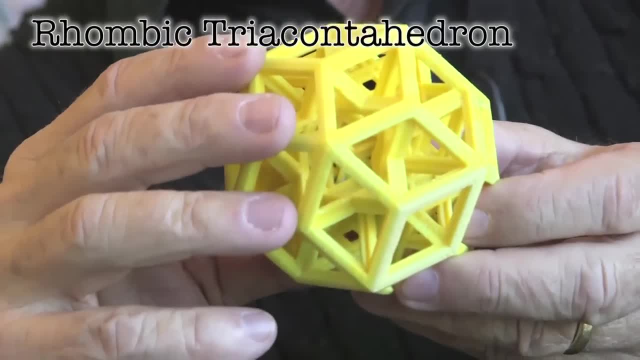 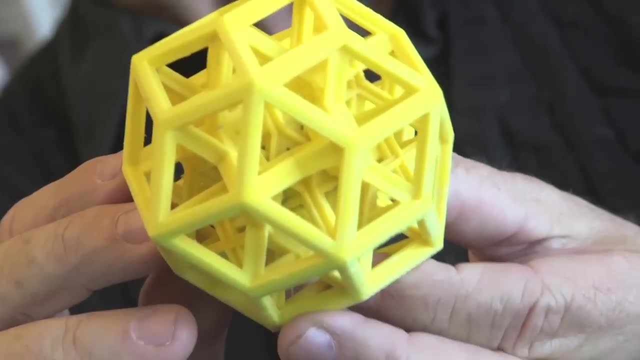 which has 30 rhombic faces on the outside, but on the inside there's a whole lot of intersecting edges going on and you may not like that. So it all depends on what you really want to get out of your model. 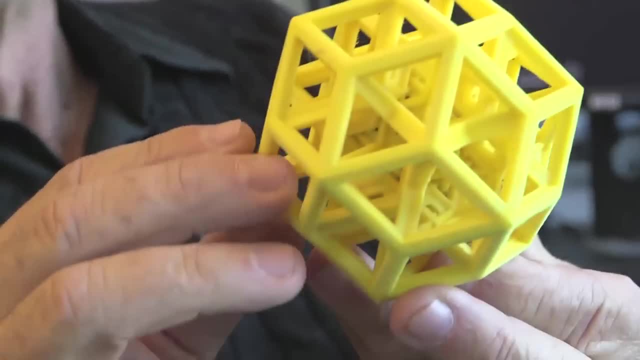 In some sense this makes a very nice soft climbing structure for children. It doesn't look very cubey though, does it? It's hard to see the cubes. Yeah, from some angles, if you look at here, it looks like an oblique kind of squashed cube. 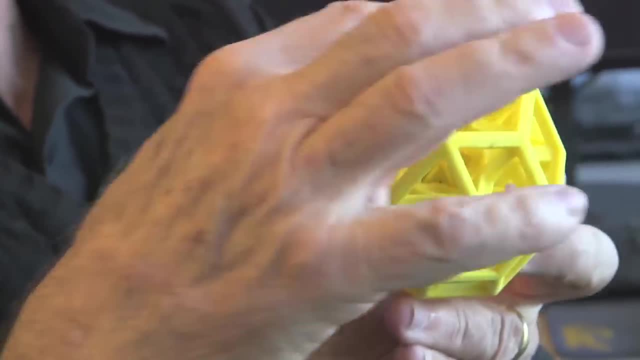 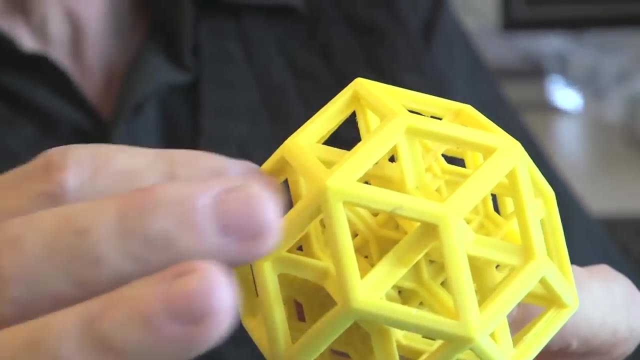 that starts as one of the cube face or a very flattened cube. You know, you have just like three faces here and then on the inside there will be another three flat faces, but they of course already intersect with edges from some of the other cubes. 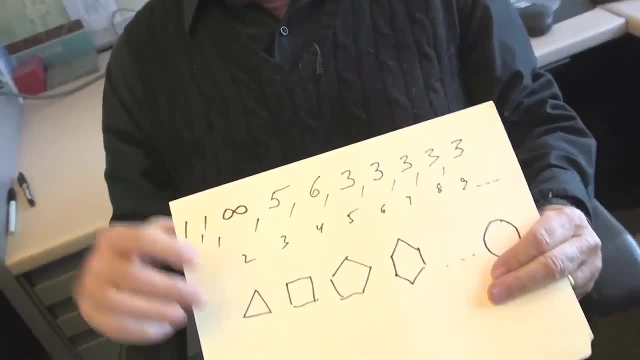 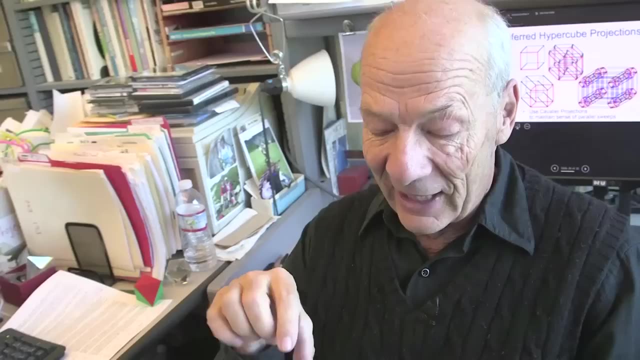 We can go cubes, all the way to infinity. That is correct. So you know, we started out with the five platonic solids, We went to the six regular polytopes in four dimensions, and after that I said three, three, three, three, three. 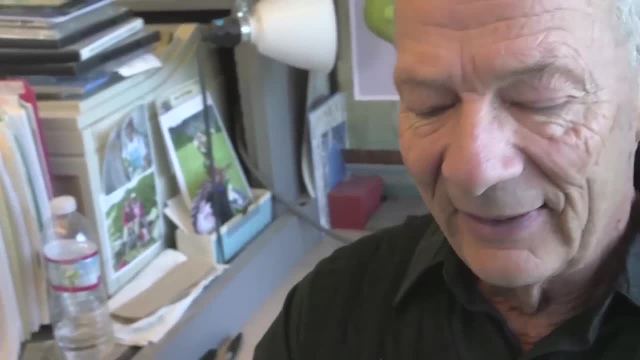 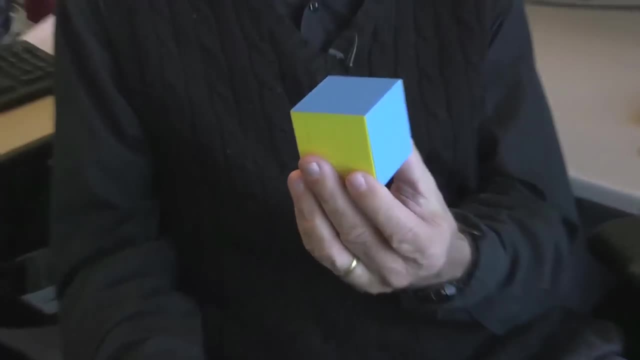 I have shown you two of those three series: the simplex series and then the measure polytope series, So there must be another one. We've seen that we can make a series of measure polytopes through all the dimensions In each one of these dimensions. 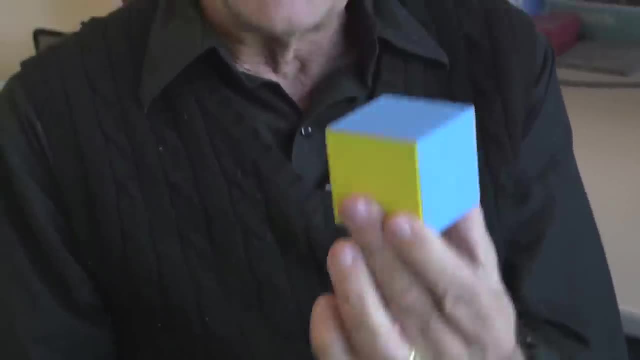 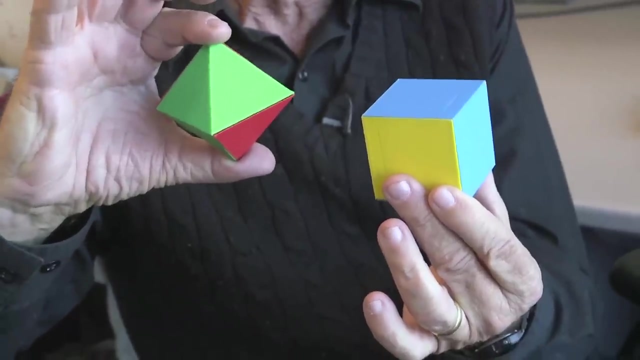 we can also form the dual, Just like in three dimensions. we have the cube and then we have its dual, which is the octahedron. If I hold it that way, you can see the top and bottom vertex in my right hand. 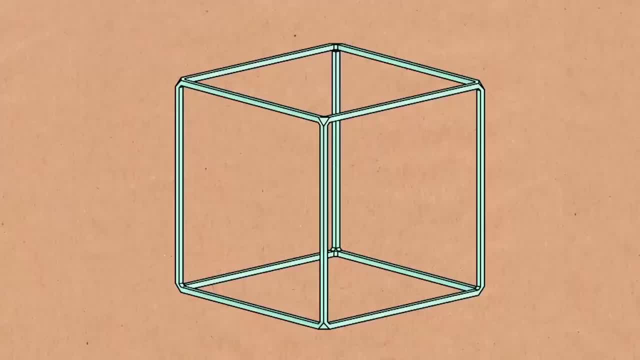 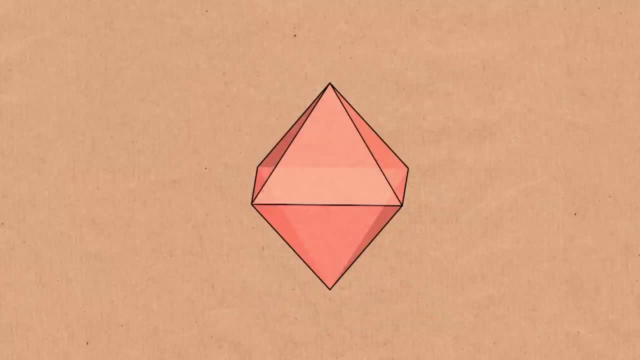 correspond to the top and bottom face in this particular cube. For each of the six faces in the cube I now have a vertex, and for each of the vertices in the cube I now have a face Like its evil twin, Yep. 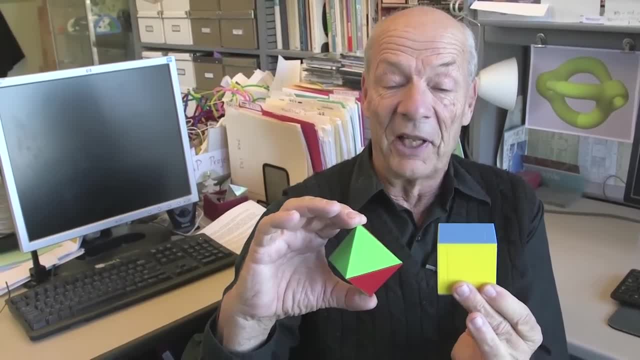 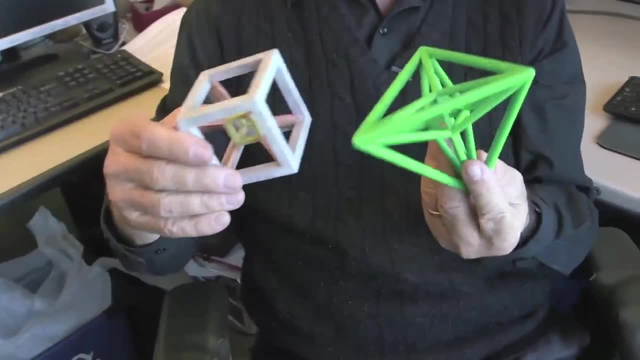 Or nice twins actually, So they're duals of one another. We also have the models that show the same relationship, not quite as obvious, in four dimensions. So here we have the measure polytope, the hypercube and, if we take the eight cubes, 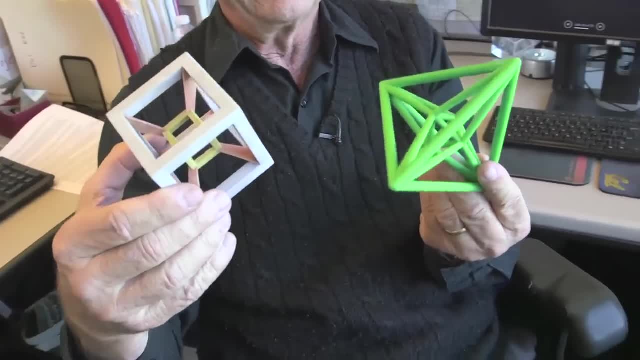 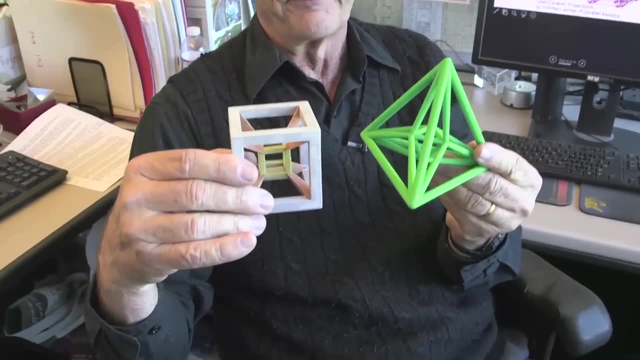 in the crust of the hypercube and replace them by eight vertices, we get the corresponding measure, polytope, which is the dual to this hypercube Evil twin, And the same principle goes on. It gets, you know, near impossible to kind of visualize. 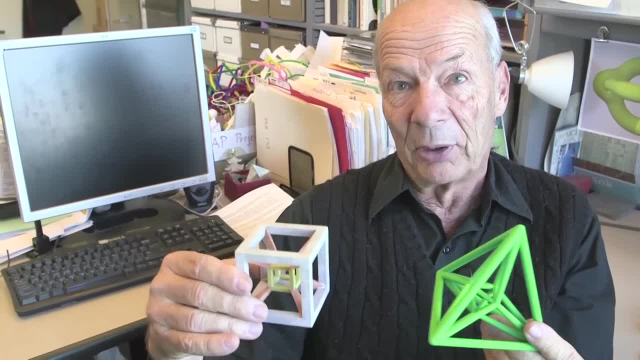 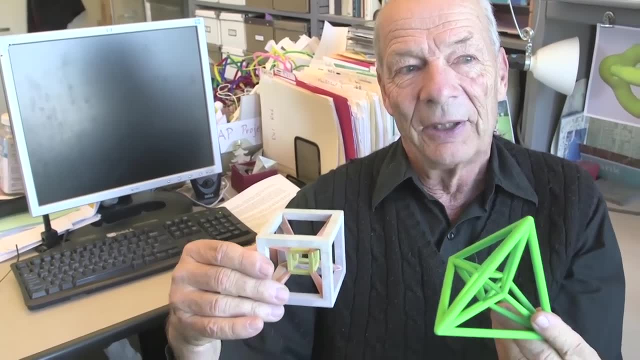 in higher dimensions. but again, every measure polytope in d dimension is made out of measure polytopes of d minus one dimension. you replace each one of those cells with a vertex at its center and connect them properly and you get the cross polytope. 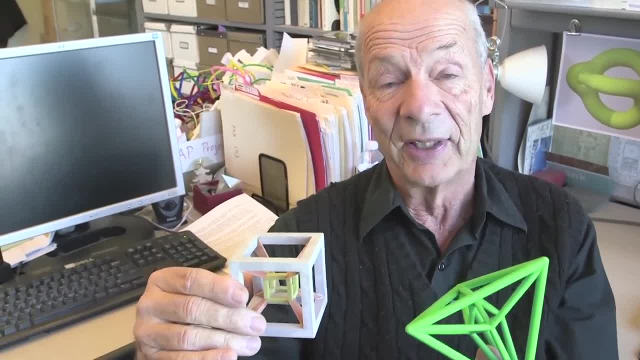 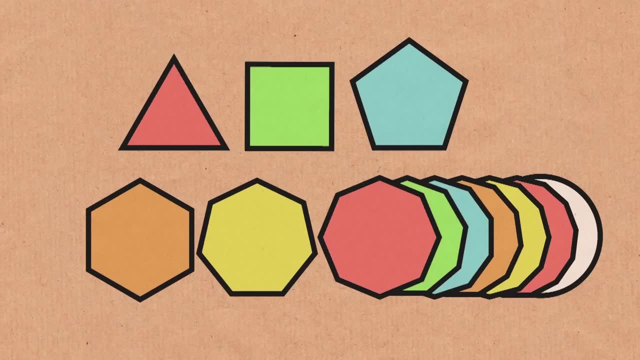 which is the dual to the measure, polytopes in any one of these dimensions, And that's the third series that we can form. Here is again our sequence. You know, we have infinitely many polygons in two dimensions. We have five platonic solids. 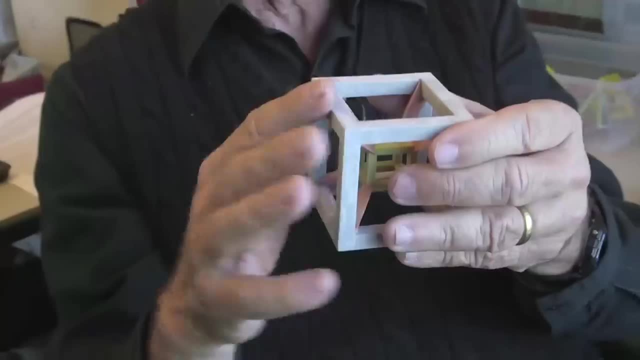 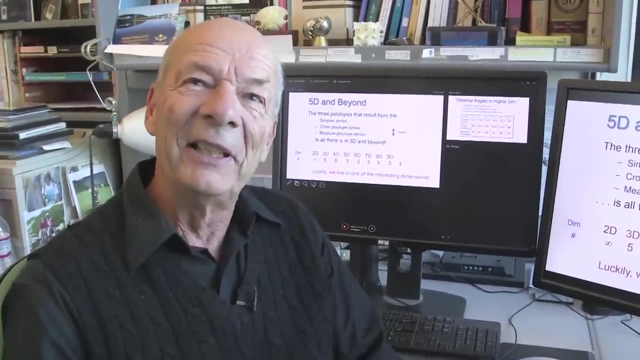 in three dimensions, six polytopes in four dimensions, and from there on it's just always only three regular polytopes. So in conclusion, I think I can say we're sort of lucky that we live in one of the two dimensions.